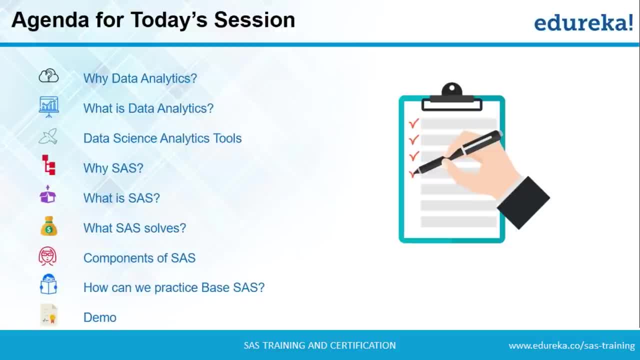 what SAS actually is. After that, we'll be seeing what SAS solves actually in the real world and then move on to the discussion, wherein we'll be seeing what are the different components of SAS and then, moving on to the topic of interest, which is base SAS. we'll see how. 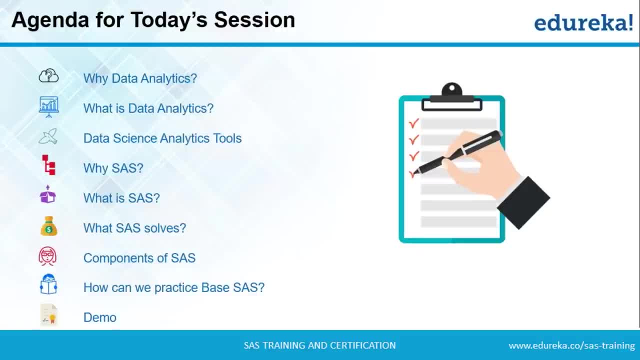 we can practice base SAS on our own. Towards the end, we'll be doing a short demo wherein we'll be getting acquainted with the SAS environment, and then we'll be talking about data analytics, And then we'll be solving simple queries and hence ending the session. 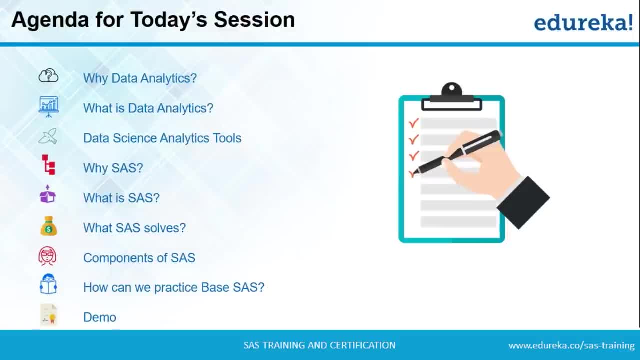 So, guys, this is our agenda for today. Are we clear with it? Alright, I'm getting confirmation. So Julen is clear, So is Saurabh Bebek is clear as well. Abhilash is clear as well. Okay, guys, since most of you are clear, let's move on to the first topic of today's discussion. 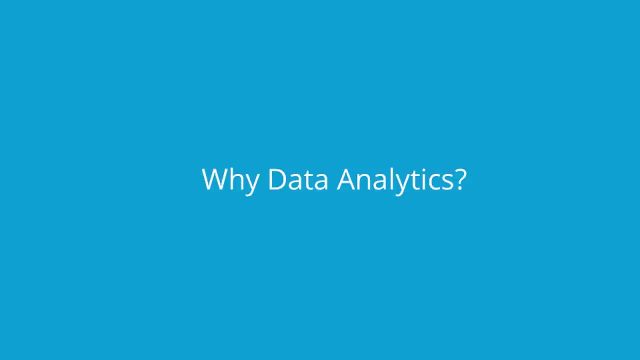 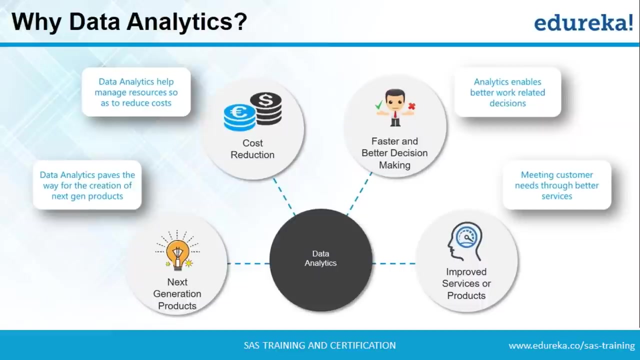 that is why data analytics. So why do we need data analytics? is the question. So data analytics is used because of these four things. So, first of all, if you are a product based company, you can come up with next generation products. So data analytics is all about data. You are 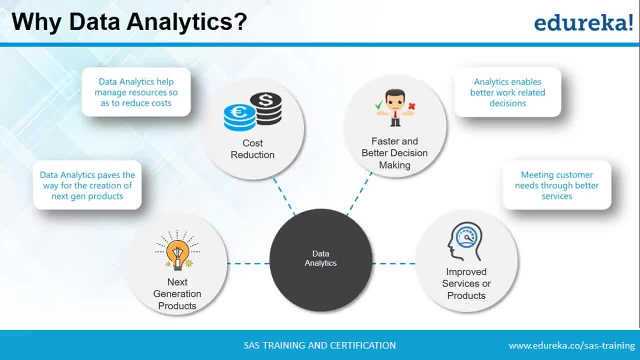 studying data. So if you have a product which has been successful in the past, but if we see the other companies whose product have been successful, you can actually study them and derive the characteristics which made those products successful. Now, based on those characteristics. 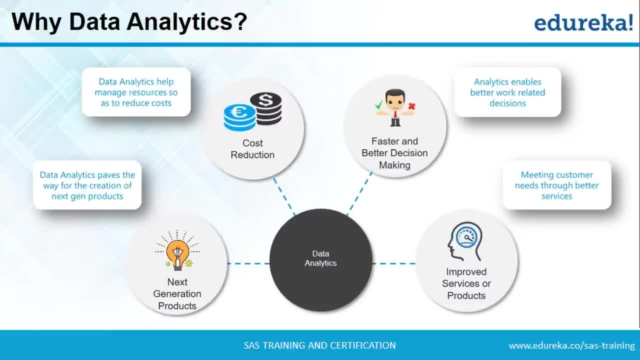 those characteristics with the new features that you're trying to implement in your product. right, You can come up with the next generation product, which will be successful and, at the same time, it will be more advanced. right Now, these features that you'll be deciding can also be decided based on the data that 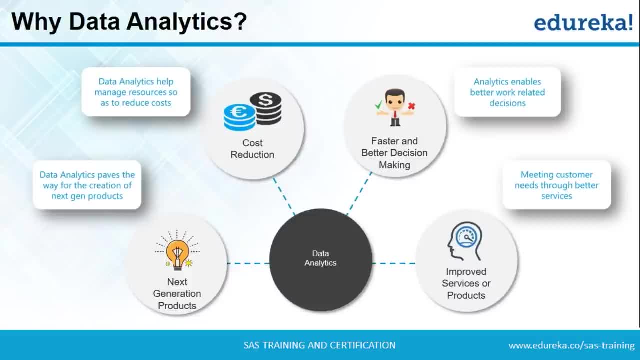 you are studying right, So say some. there was some product which was launched last. last year there was some mobile phone right And on the basis of the user feedback you get to know, okay, so in terms of usability, it is better to have. 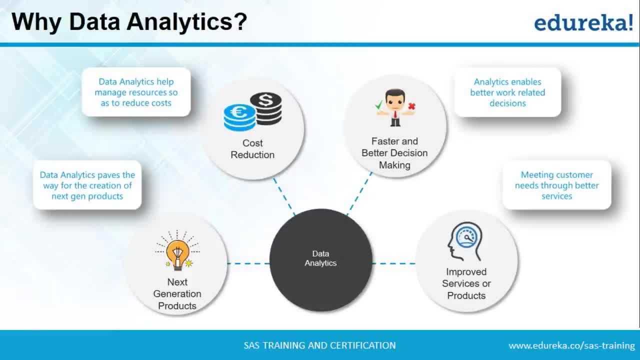 the fingerprint sensor on the front rather than the back right. So you take that feedback, implement in your own product and come up with the product which is not only usable but has more features, and hence it becomes a next-generation product. Having said that, let's move on to the second property. 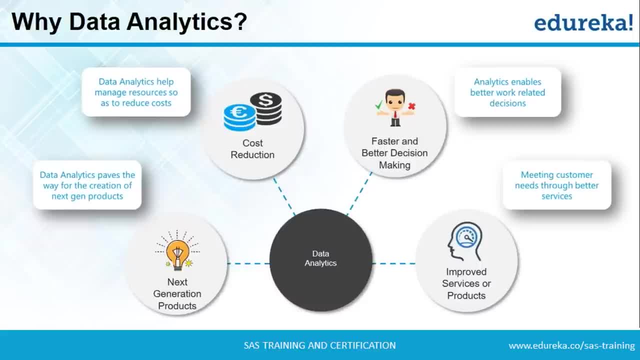 which is cost reduction- right. So you can actually study the way you have been spending on your projects, right. And then you can actually come up with a plan wherein you can see: okay, I went wrong here by investing more money in this thing, or I spend more money on this thing and I didn't get any results, right. 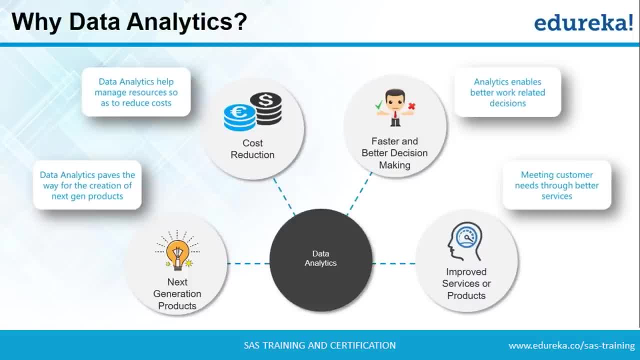 So it's better not to invest money over there. You can do all these kind of analysis and hence reduce costs on your project right. Or else you can also study products from different companies or other companies who have actually released their that product at a lesser price, so you can see what made them minimize the. 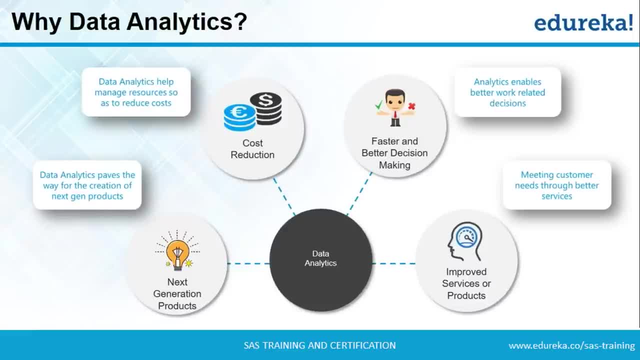 costs in their production. right, You can implement that in your own production line and hence reduce costs of your projects. Then you have a better decision-making process. So data analytics basically provides you with facts. it provides you with a path to whatever you are trying to achieve, right. 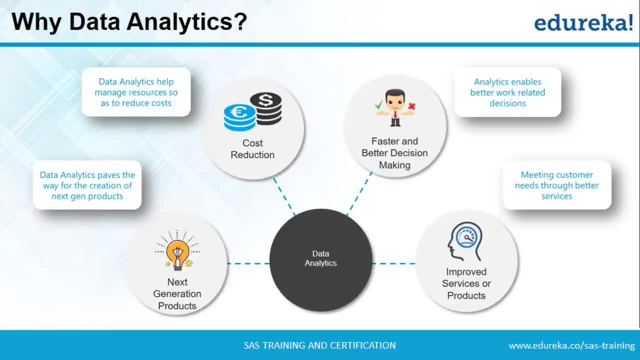 And when you have a path and you have facts presented in front of you- mathematical facts, mathematical proven facts- right? So your decision-making actually becomes easier because you obviously want yourself to be succeeding, right? So if you want yourself to be succeeding and you see a way, okay, so, 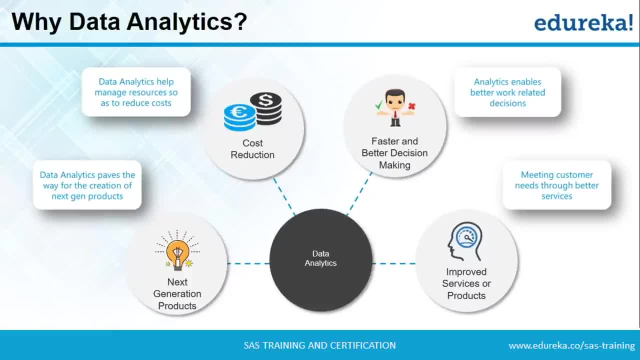 this is the way that data analytics, or this is the way that trends, have shown me, so let me go this way, So your decision-making actually becomes easier. right, And hence data analytics plays a big role here And, towards the end, it actually improves the service of production. 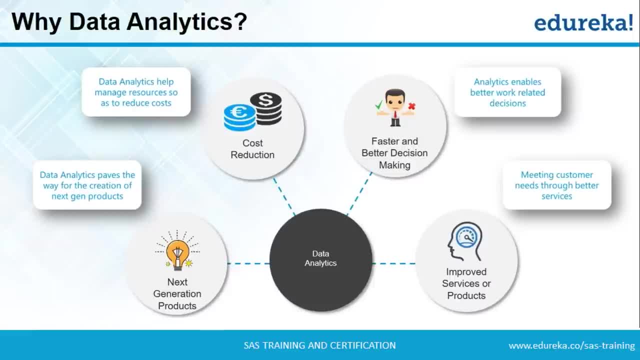 And if you're allowed to do your own decision-making now, then data analytics is not required because it just becomes easier to then certolize the products that your company serves. right When you are producing the next generation products. you're offering your product at a lower price and you're also doing the right thing by following a particular path which your friends have shown. it obviously improves your service or product because it is more efficient. now It is more relatable to your customer because you have studied the customer feedback right. So it is more relatable to your customer and your customer is more happy with your product. So it greatly 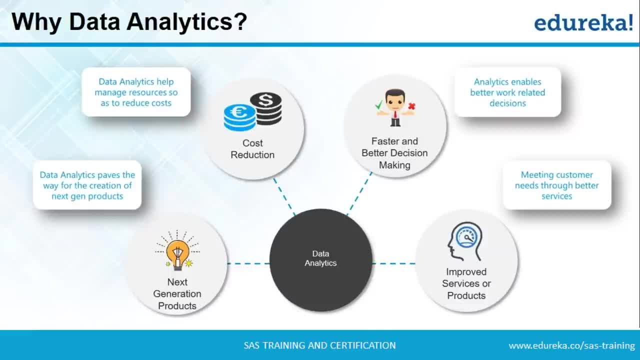 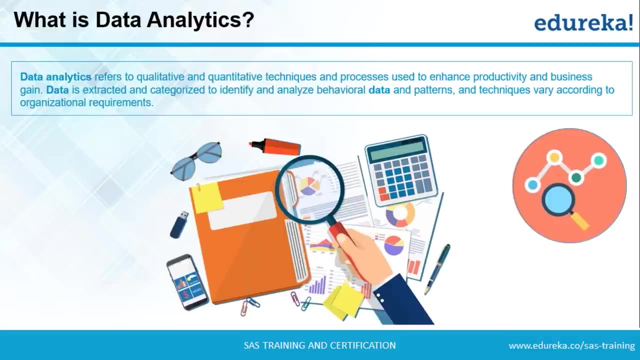 improves your service and products. Having said that, this is why data analytics is actually important, right? So we have discussed why do we need data analytics, and let's now move on to the part where we will discuss what data analytics actually is. So data analytics refers to the qualitative and 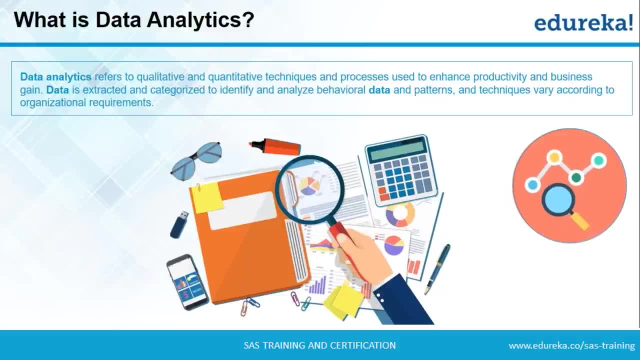 quantitative techniques. So qualitative basically means that you are obviously increasing the quality of your product, using trends, using techniques. Quantitative means you're employing formulas, you're employing statistic facts to come up with figures, which actually gives an insight on your product, right? So you employ these quantitative and qualitative techniques. 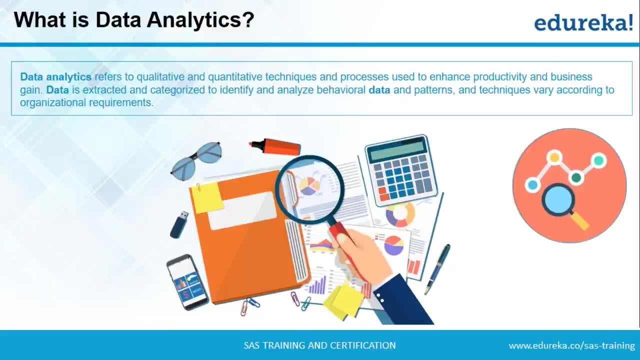 or processes and which are then used to enhance the productivity and the business game right. So, obviously, if you improve the quality of your product and in terms of quantity, if you say you increase the bandwidth of your product, say you were making three hundred products previously and you're now with improved efficiency, you can now 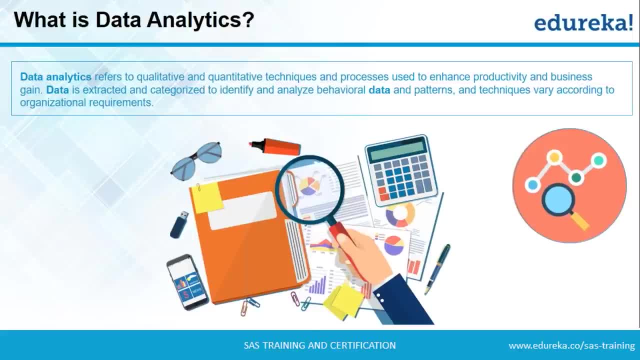 make six hundred products right. So you are obviously increasing or enhancing the productivity and obviously, since your productivity has increased, your business gains increase as well. right Now, data analytics is not magic guys. it's purely science. it's based on science and it is based on data, The most important. 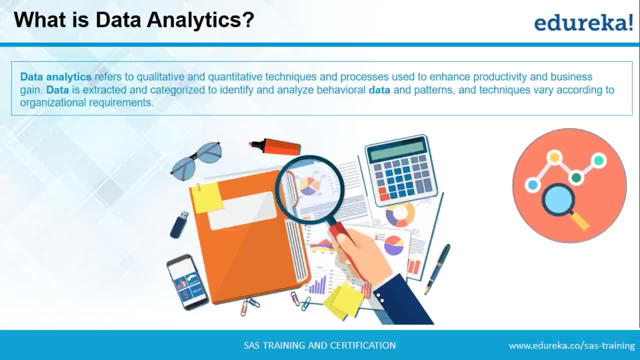 ingredient in analytics is data. right, So now, where is that data coming from? So that data is actually extracted from your feedback, from social media? right, So you can extract data from them and then categorize it and then, hence, analyze it on behavioral aspects. You can. 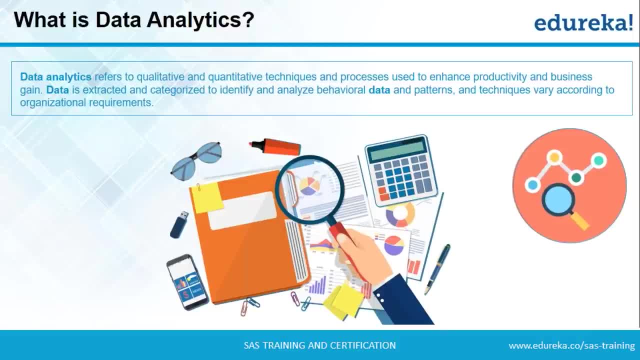 actually see, or you can apply sentiment analysis on it and see how is the feedback coming from customers on your particular product and you can actually categorize the negative feedbacks and see what are those users saying. what did they find wrong, wrong in the product or what more do they want in the product and hence implement that. 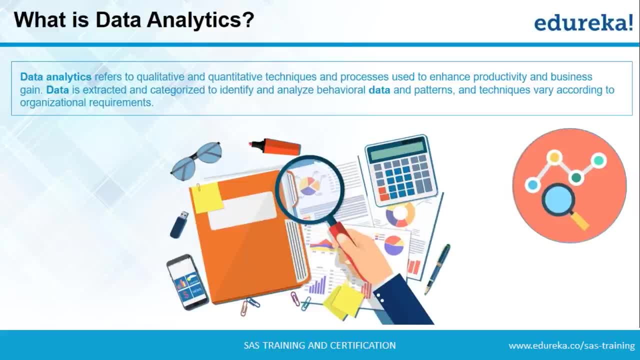 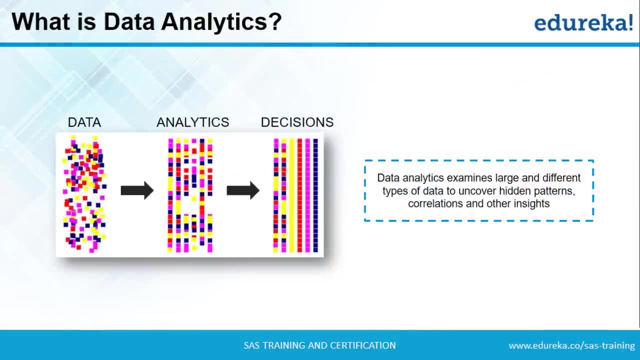 in your next release. Okay, so this is what data analytics is, guys. So now, how? like I said, so, data analytics is not magic, right? so let me give you an example for that. So, if you imagine data, because data is random, alright, so data has no structure. 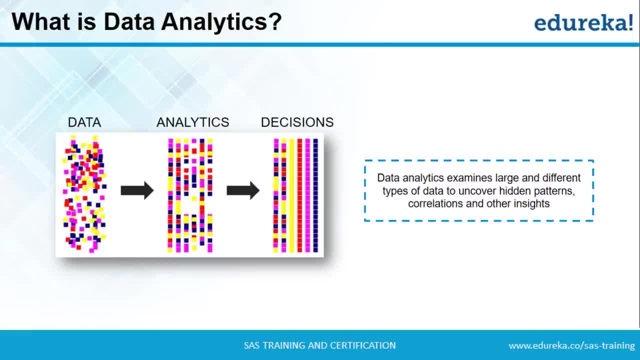 So data, when you provide structure to the data, that is what analytics is. So this is your data. it is all unstructured, but with the help of some tools, You come up with a structured kind of an array, and this is what analytics is. 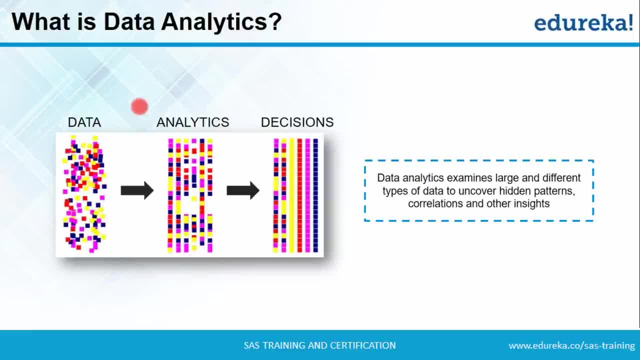 Now your job is to analyze, or to read the facts that analytics provides you, and then come up with decisions. right, then you come up with decisions and then it becomes all sorted. So this is a large data, so maybe this is something that you have taken from social. 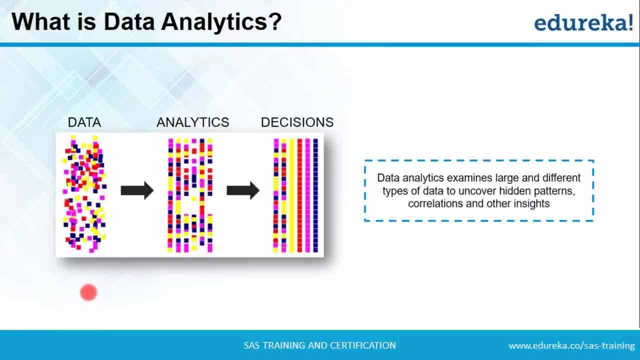 media you have taken from different sources, and all of that you have dumped in one particular place. So now you want to analyze it, right, so you would employ an analytics tool. that analytics tool will actually try to read this data and make sense out of it, and this is what it does. 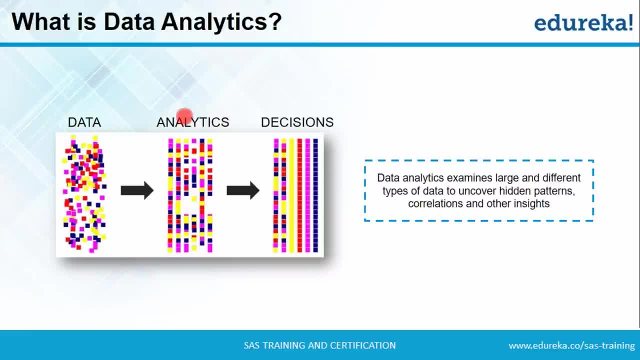 It makes sense out of it, it categorizes it, and then it's your job to actually analyze it, so using different techniques. So once you analyze it, based on the results, you come up with decisions. right, and this is what the decisions look like. 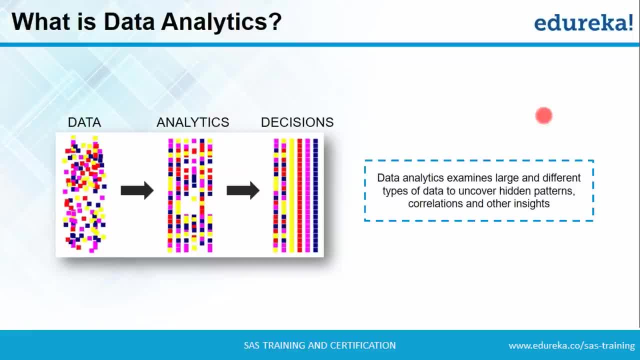 This is the sorted form of your data, right? So this is how data analytics is actually used: to solve, or to come up with predictions, or to come up with paths that will lead you to success. Having said that, I was talking about tools that can be used to perform data analytics. 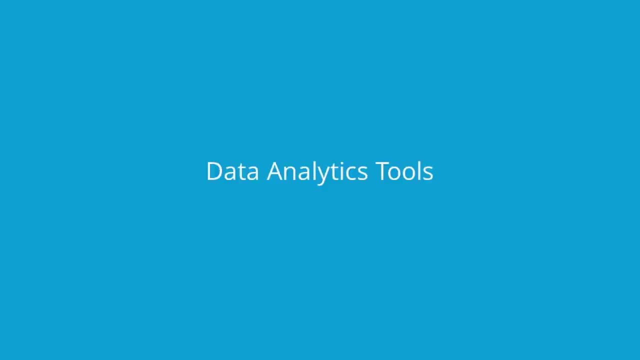 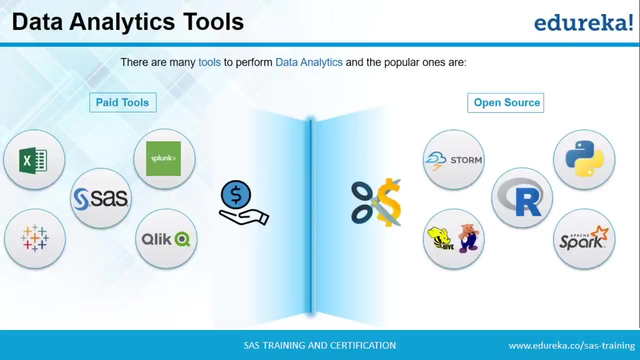 So let's move on and understand what are the different tools which can be used. So data analytics tools are of two kinds. one is the paid kind, wherein you have to pay for the software or the tool that you are trying to use, and one is open source. 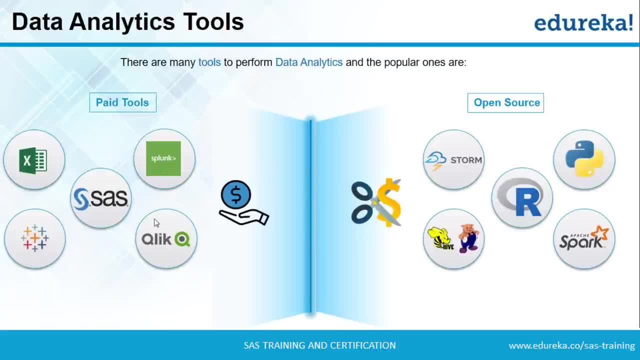 Now in paid tools, you have Excel, you have Splunk, you have ClickView, you have Tableau and you have SaaS. In the open source part, you have R, you have Pighive, you have SparkR, you have Python. 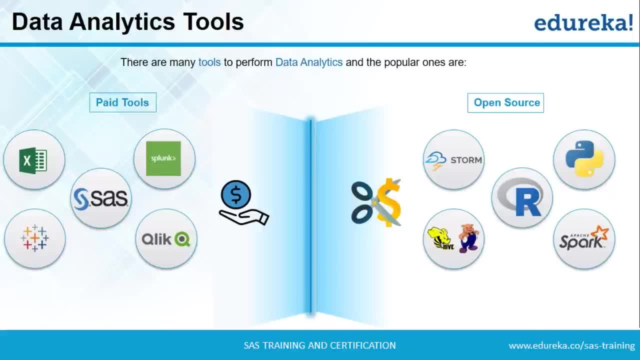 and other tools as well. Now, today, we are going to discuss SaaS, right? So why have we chosen SaaS out of all these different tools? What is so special in SaaS? Let's discuss that. So why SaaS? Now, we are using SaaS because of these reasons. 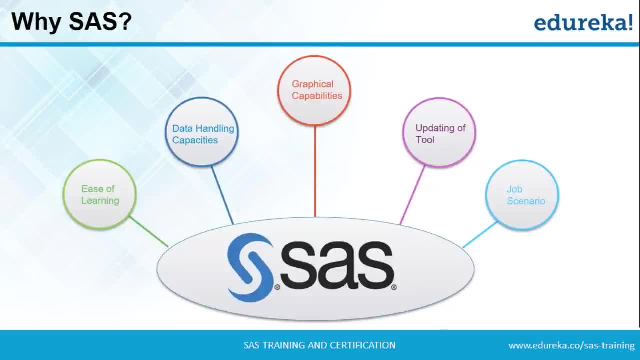 So it is easy to learn. and because of data handling capacities, graphical capabilities, updating of tool and job scenarios, Let's look at each of these one by one. So let's talk about ease of learning first. So SaaS is very easy to learn, guys. 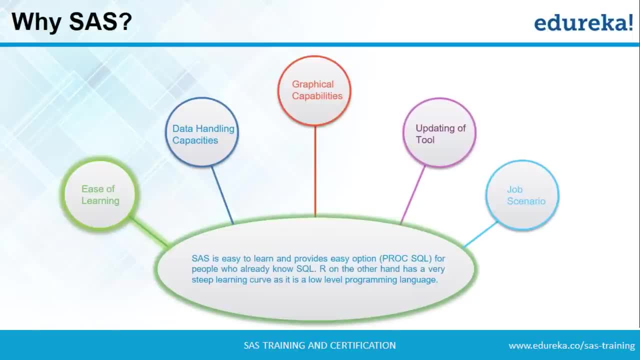 It basically follows procedural SQL language and people who have an experience in SQL will actually be able to relate to this language more right. And if you compare it with R, which is an open source language, It is a very steep learning curve, as in it is very difficult to learn R because of the 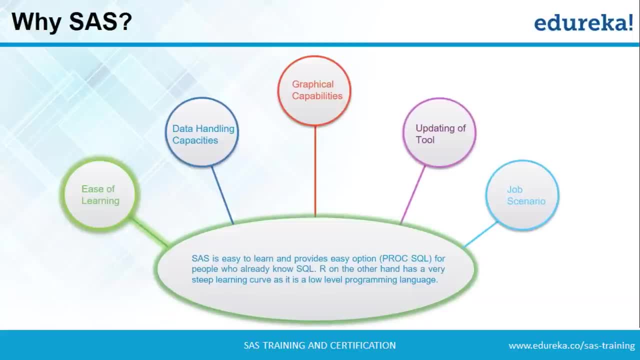 language, which is there because it is completely new. it is not related to any technology that you are using right now. It is not relatable, right, And that is why it becomes a little difficult to learn R than it is difficult to learn SaaS. 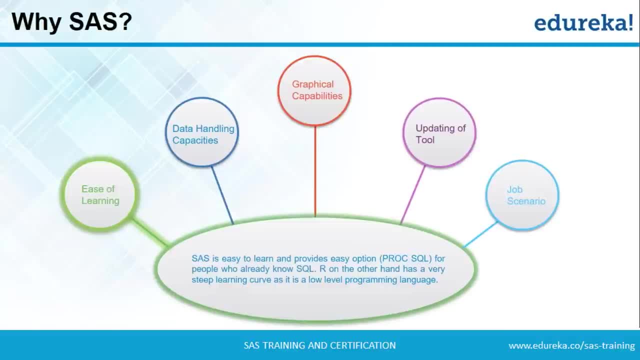 So SaaS is comparatively more easier than learning R, and that is the reason people are more inclined towards SaaS when they enter into the data analytics field. Since you guys are beginners- right Beginners- people like you would prefer SaaS more than R, because SaaS is more easy to learn. 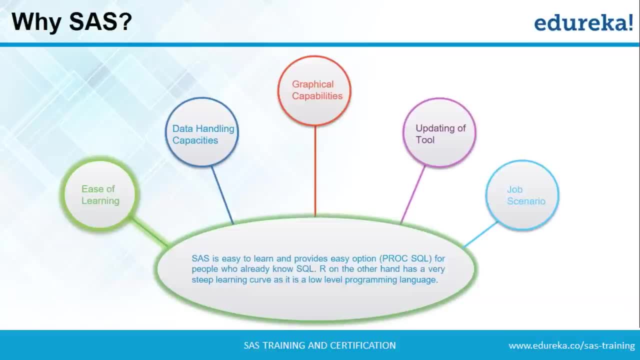 and hence it will be more easier to get into this career by learning SaaS. Having said that, so ease of learning is the first reason. The next reason is data handling capabilities- right? So when we talk about data handling capabilities, SaaS is in par with R and Python when it comes. 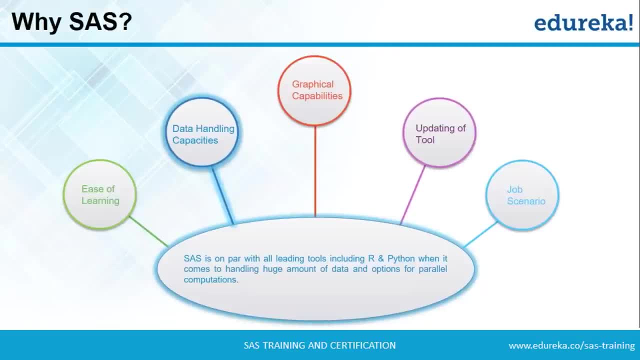 to handling huge amount of data, right? So it performs at par with R and Python, So it's not like in open source: You have a tool. It's better than SaaS, right? So SaaS is in par with R and Python, which are open source, in terms of handling the size. 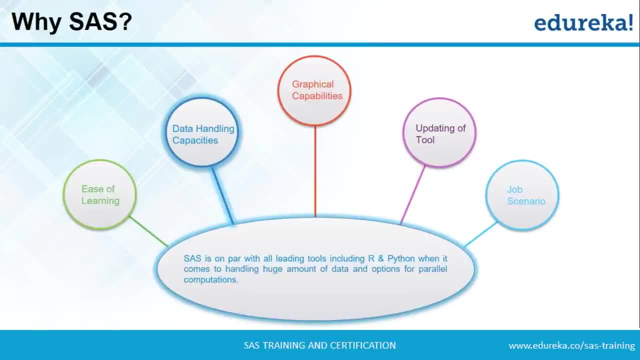 of data that we want, right? So if there's a huge set of data, so SaaS can handle that efficiently. Moving on, let's talk about the graphical capabilities. So, using SaaS, you can come up with various graphs or various types of visualization tools. 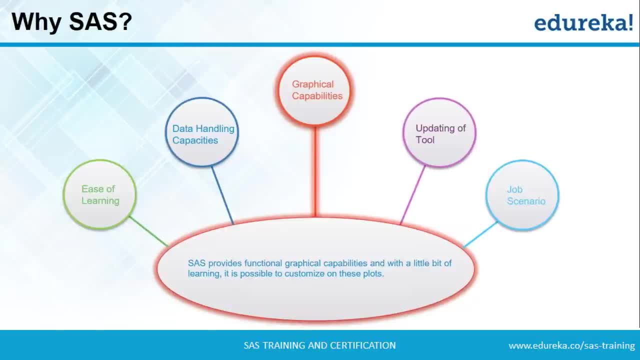 or graphs so that you can study your data more quickly, Because it gives you more insights when you're going with the visualization way than actually studying the data right. So with a little bit of learning, it is possible. So by learning only a few commands, you can actually come up with good graphs, which gives 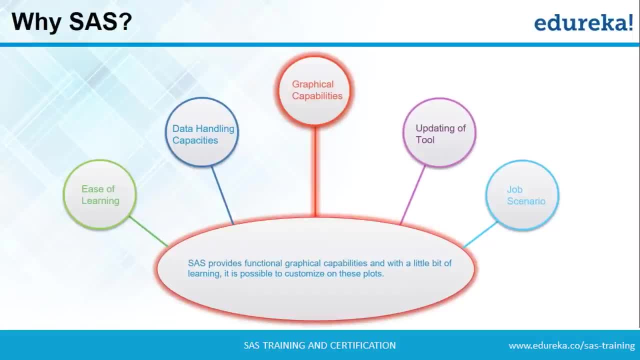 you good insights into your data, right? So the graphical capabilities is also a reason. Then comes updating of tools. Now when we talk about open source guys, so open source, you have to rely on the community to come up with the next version, right? 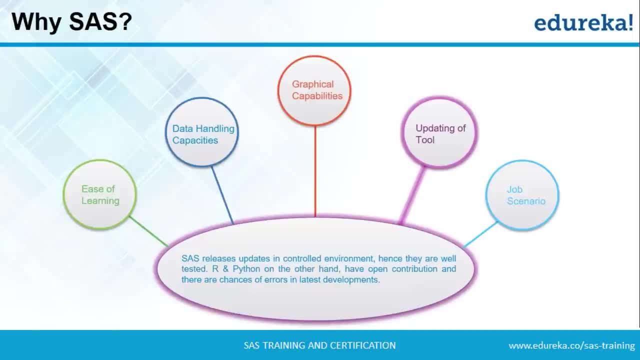 But with SaaS it is not. It's just not like that. So whenever they feel that there's a new feature coming up, right. So since SaaS is a paid tool, it's a proper company, right. So their updations are very systematic, right. 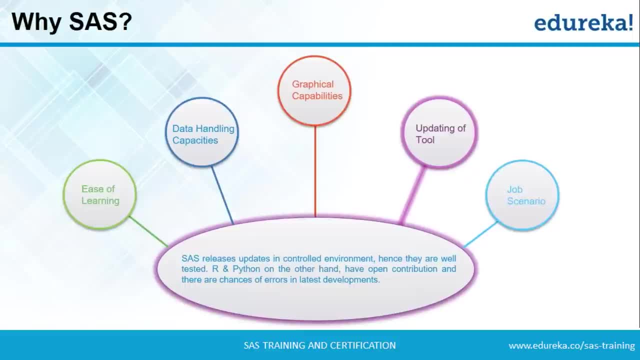 So they come up with new features now and then They come up with new ways of implementing techniques, and when they say new ways, they're actually making it more easier with every release of theirs. When you talk about R, R is not that frequent- or when you talk about other open source tools, 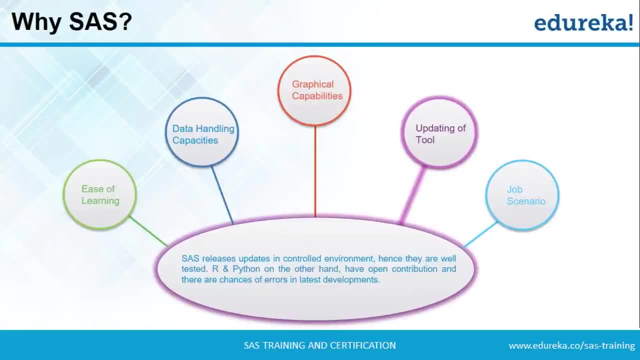 they in terms of using or in terms of their updations. I'll not say they're not updated at all. They are, but they are updated at a very low pace, right, And we, since we are working in businesses, we want the best of the best, right. 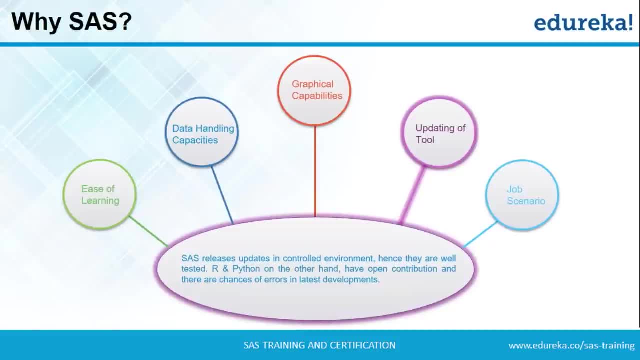 And if you have a tool which is upgraded according to the latest technologies which are out there, it becomes more easier for us to implement that technology, right? Having said that, so updation of tools is also a reason. And then comes the next step, right. 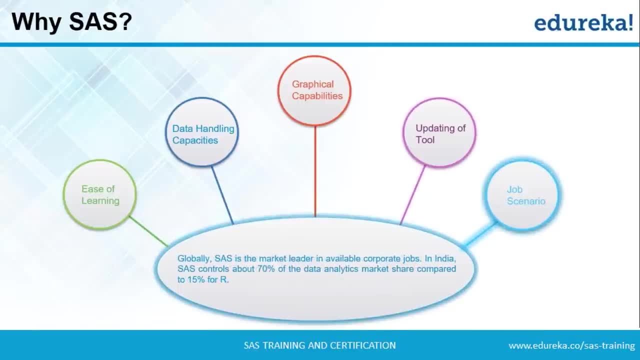 So the next step is to come up with a new tool. So the next step is to come up with a new tool. So the next step is to come up with a new tool. And then comes job scenario. So if you talk about our country, India, so the companies which are using SAS are 70%. 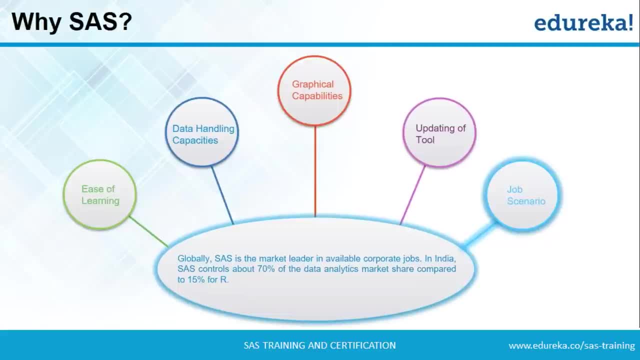 So 70% of the data analytics population is using SAS, as compared to the 15% population which are still stuck on R right? So if you're learning SAS, you have a better opportunity to be employed in the data analytics industry than if you're learning R, because R has a comparatively lesser community, or? 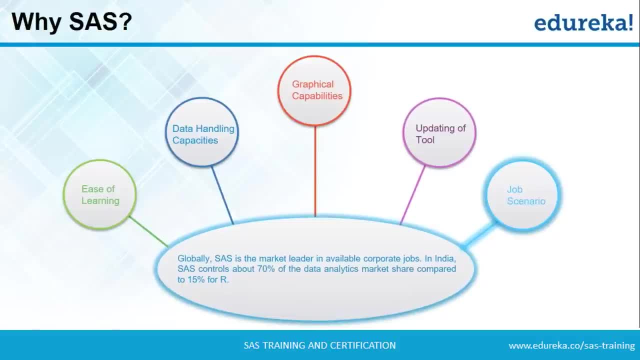 there are lesser businesses which are actually implementing R for data analytics in today's world right. So these were the reasons, and these are the reasons that people are actually preferring SAS over any other language, because first it is very easy to learn, Then the data handling capabilities are at par with the other languages. 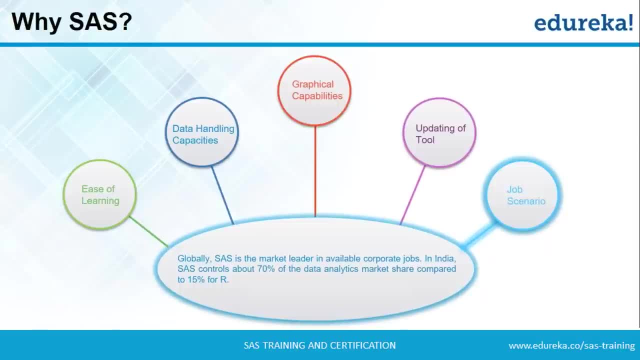 The graphical capabilities are also there and they are very easy to learn again. And then the updates are pretty frequent And the job scenario is also very easy to learn Right. So the job scenario is cool as well. So if you're learning SAS, you increase your probability of being employed as a data analyst. 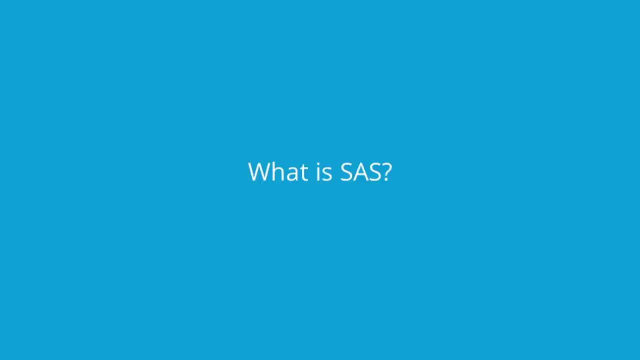 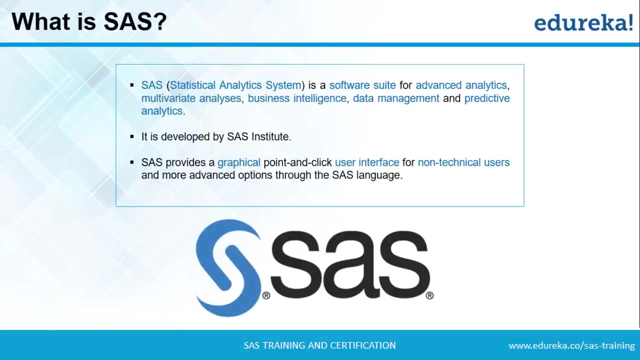 right. So this is why SAS is preferred. Moving on now we know why we picked up SAS. So what is the reason behind you guys learning SAS right? Now let's discuss what SAS actually is. right? So SAS is a software suite, right? 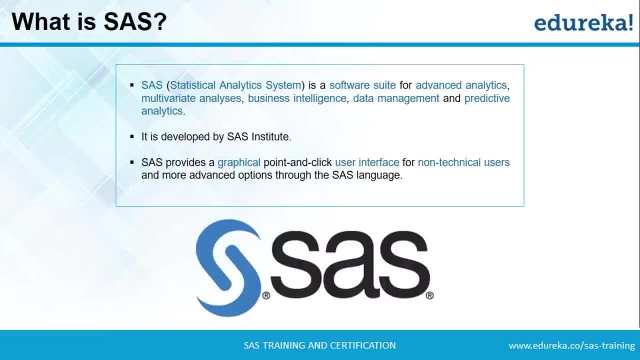 So it's a suite which contains a different kind of tool that has a lot of components right. It deals with different kind of things And it is used to do advanced analytics, multivariate analysis, business intelligence, data management and predictive analytics. 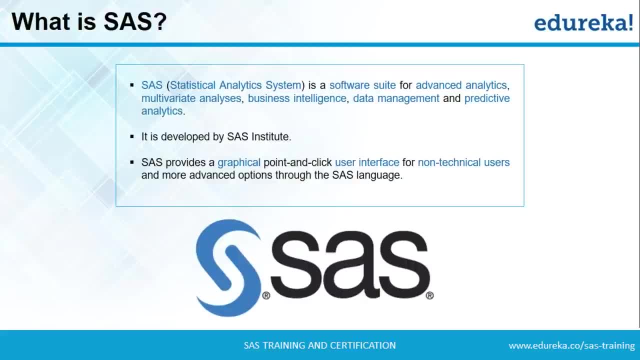 We'll discuss each of these in the next slide, So let's check it off as of now. Then it was developed by the SAS Institute way early- I think in the 1980s or the 70s- And since then it's been using. 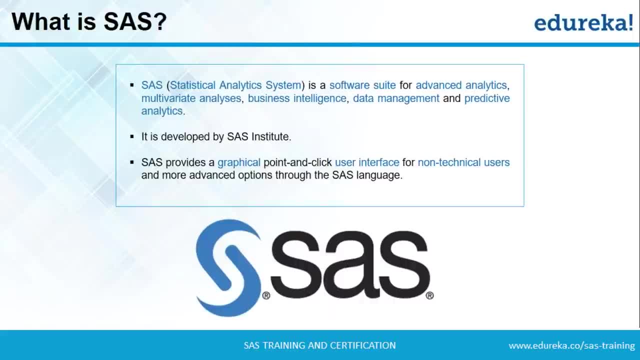 And one more reason that people tend to stick on to SAS and not go somewhere else: SAS is a software suite. SAS is a software suite. SAS is a software suite, And one of the reasons why I'm talking about SAS and not anywhere else is because SAS came. 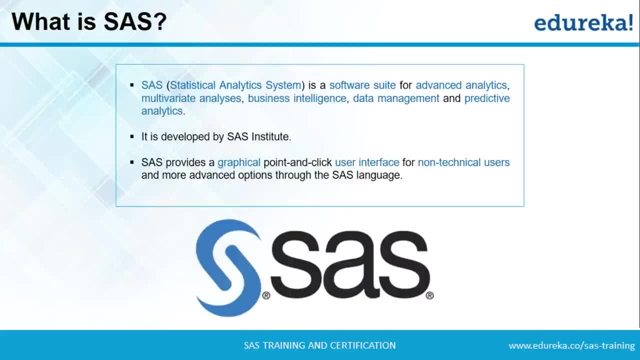 way earlier, guys, right. And now, when the systems, or when the companies have already implemented their systems in SAS, moving on to some other language becomes very expensive because they have to actually shift or they have to migrate from their legacy systems to the new systems, right. 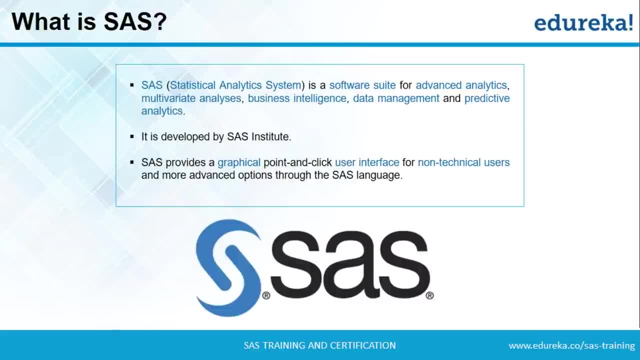 So the underlying architecture, the coding, everything will change. So when I say underlying architecture, I basically mean when you're migrating your data onto a new system system, you have to architect it again the way, because your data is now acquainted with this architecture of SAS, right? so you have to remodel everything. 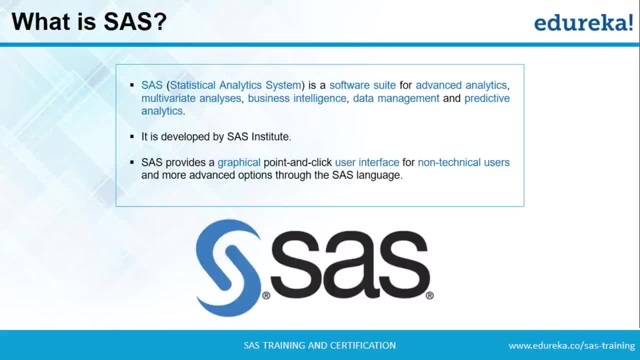 and come up with a new infrastructure, and also your employees. they are trained with the way that things happen in SAS, so you have to again train your employees for the new technology that you are implementing right, and hence the costs go up, and that is the reason people tend to stick on to SAS rather than moving. 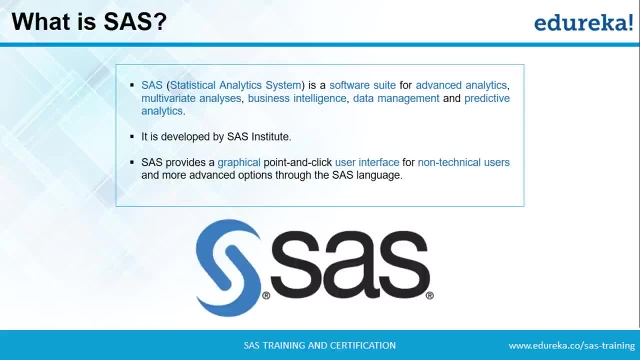 ahead. okay, so let's move on. so it was developed by the SAS Institute way early, and then it provides a graphical point-and-click user interface. the graphs or the visualization tools which are there in SAS are easily accessible, right? so you don't have to dig deep, you don't have to do a lot of research on. 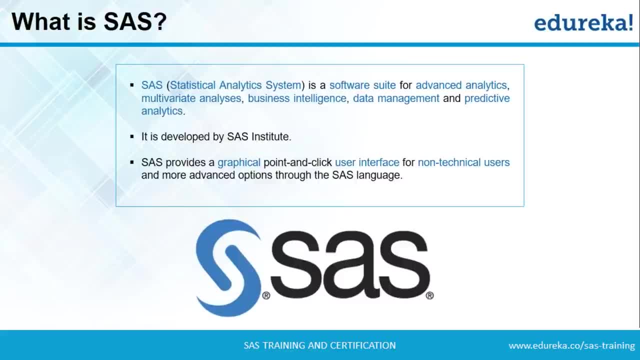 the commands which are there, it is very easy to access and with a point-and-click user interface, even for non-technical users it becomes very easy to use, right? so if I am say, I am from a technical background, so if you're, you guys, any of you, from a 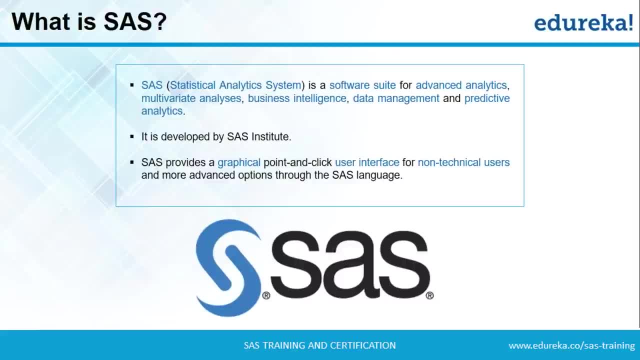 non-technical background, SAS will make sense for you as well. right, so it will not be difficult for you to actually use SAS because of the interface or because of the UI or because of its user friendliness. right so this was about SAS, guys. so, like I said, it is a software suite for a different kind of things. 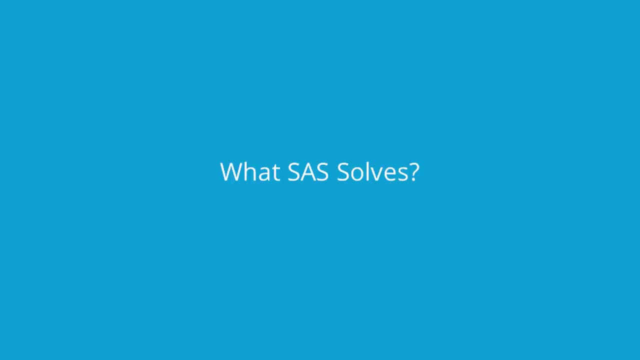 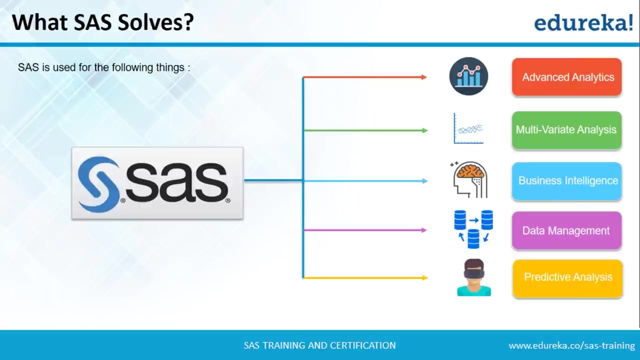 let's discuss these things. so these are the things which SAS actually solves, right? so let's see. so SAS is used to do advanced analytics, it is used to do multivariate analysis, it is used for business intelligence, it is used for data management and it is used for predictive analysis. now let's discuss. 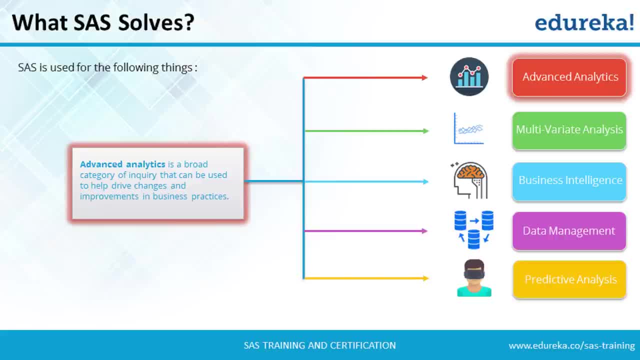 each of these one by one. so, first, what is advanced analytics? right, so it is a broad category of inquiry that can be used to help write changes and improvements in business practices, right? so, like I said, it is just like data analytics, so it is just an advanced form of data analytics. 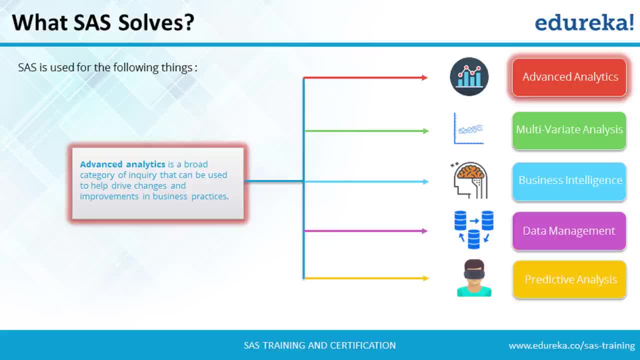 wherein you use more sophisticated techniques and you come up with the insights which can help change and improve your business practices. right? so this is what advanced analytics is all about. then you have the multivariate analysis. so when you have, when you're doing analysis, you actually depend on some. 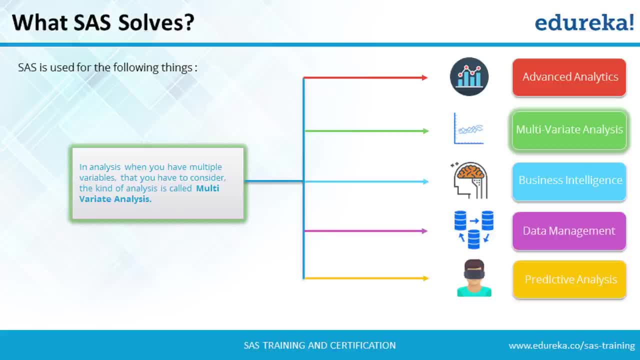 variables, right, So some factors which actually are causing a change in your model. So when you have a lot of factors involved, like if you have, say, like when I talk about the capacity, the engine capacity of a car, it is based on a lot. 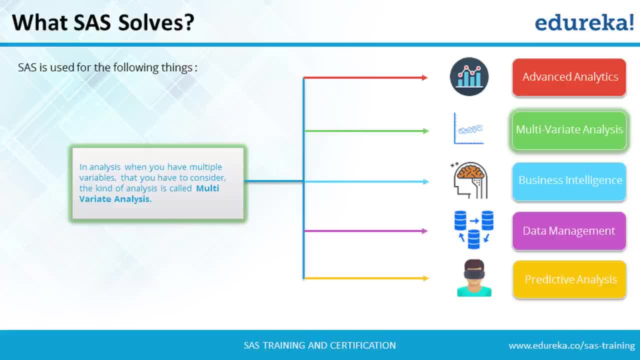 of things. It's based on the weight of the car, it is based on the dimensions of the car. it is also based on the terrain that it is meant for. So when you look at all these things, you come up and say, okay, so this is the engine capacity that. 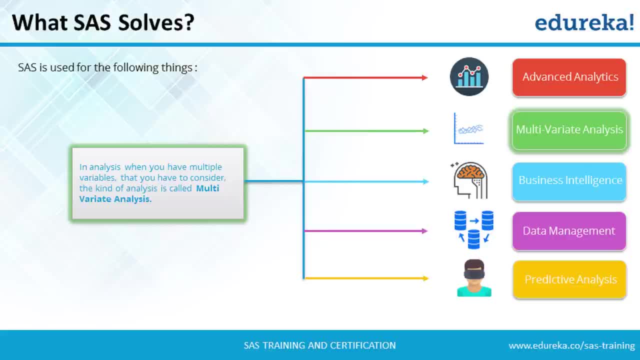 this car should have right. So you're taking into a lot of things. you're taken into a lot of variables. Similar is the case with SAS as well. So SAS actually is used where you have a lot of variables. So I just took three variables. 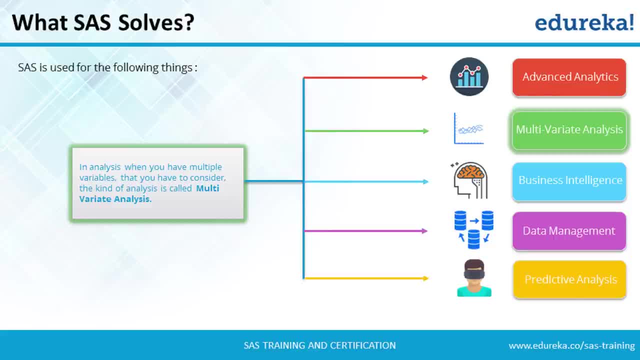 that could be around 15 or 20 or 35 or 40 variables, right? So when you have these many variables and you're trying to make a decision based on all these variables, it actually becomes a cumbersome task. but when you have SAS, you don't have to worry about anything because it is. 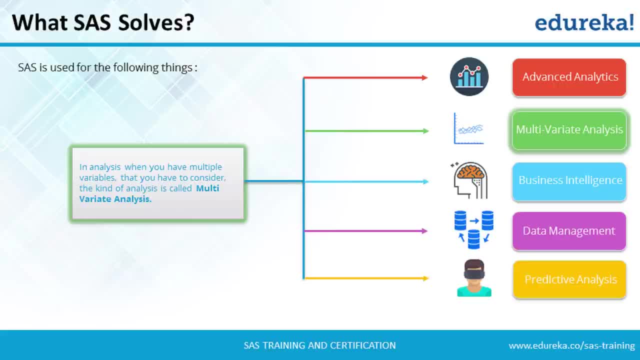 used in this software, where it is efficient in these kind of analysis. Moving on, then you have the business intelligence topic. So what is business intelligence? So it refers to technologies, application and practices for the collection, integration, analysis and presentation of business information, right? So it actually refers to the 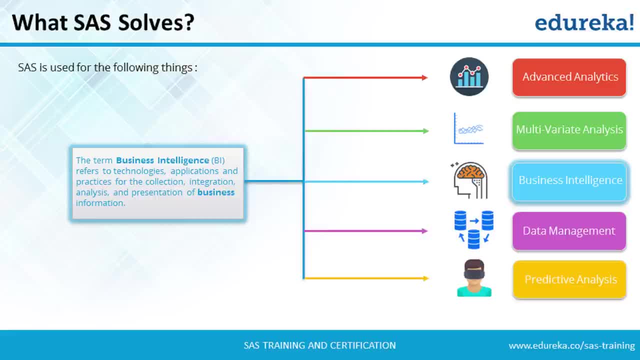 techniques. it refers to the practices that can be used to improve your business, that can be used to help your business to improve, right. So whenever you have something going on in your business and you want to understand how that business, how my business- is doing, so that involves some techniques, right. 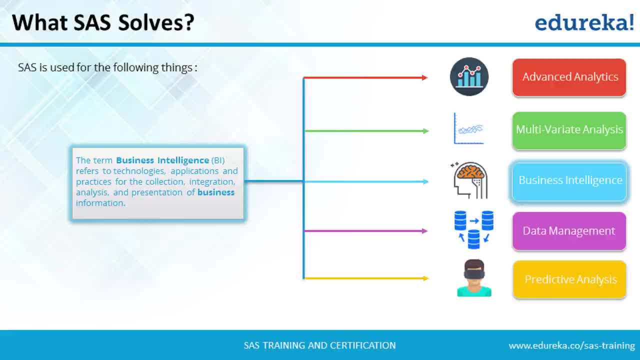 So business intelligence basically means that you are actually referring to technologies, you are actually referring to applications, you are actually referring to the practices, which leads to collection, integration, analysis and the presentation of the business information that you want to understand, right? So 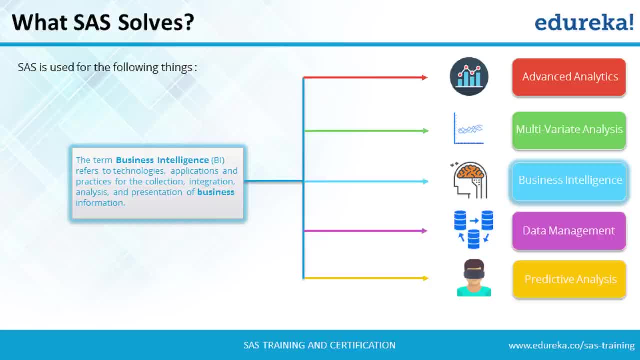 using tools, you do this, and SaaS is an all-in-one for this. So using SaaS can be a great topic of discussion and knows-how, and so it's needed to еllwous Mayo When you remember your synonyms, And so it's a key thing to remember. So you 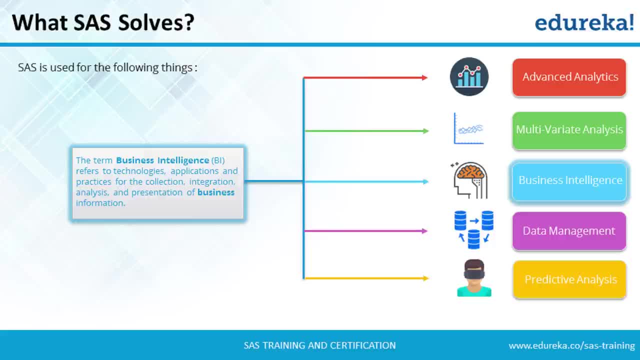 SaaS. you can actually understand, you can actually look into your business information. If you made breakthrough in sales right in the past month and you want to understand what actually made this breakthrough or what actually made this last month so successful, you can actually lead on to or you can actually. 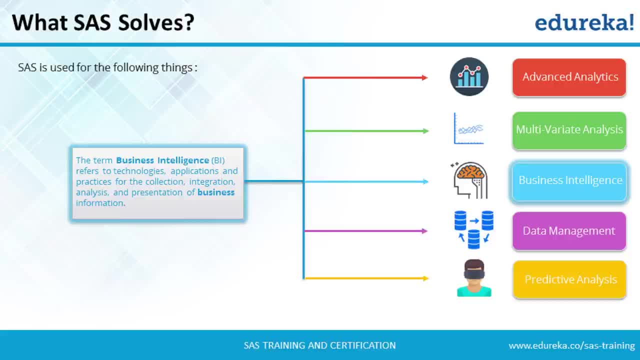 incline on your business intelligence tools, which will give you insights on to what is actually happening in your business. Okay, moving on, you have data management. So data management basically means how well you can manage your data. So with the help of architecture, with the help of policies, practices and 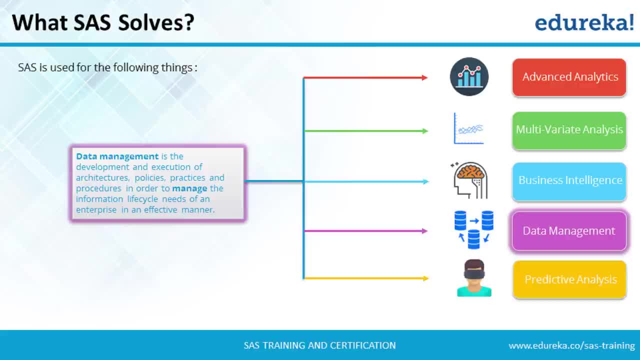 procedures, you'll be actually managing your data efficiently Now with SAS. you have all these things in place. You have proper procedures, you have proper architectures, you have proper practices, which are coded in SAS, using which you can manage your data more efficiently than some other tool. Alright, 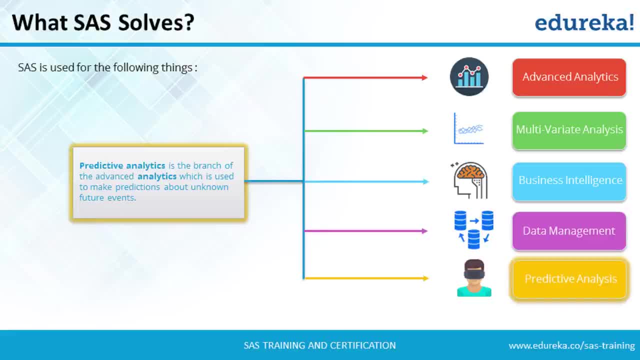 and then you have predictive analysis as well. So predictive analysis is basically a part of advanced analytics, wherein you actually foresee what will happen if these are the inputs that I give right. So predictive analysis is basically used for unknown events. So if you want to know, if I follow this path, what will be, 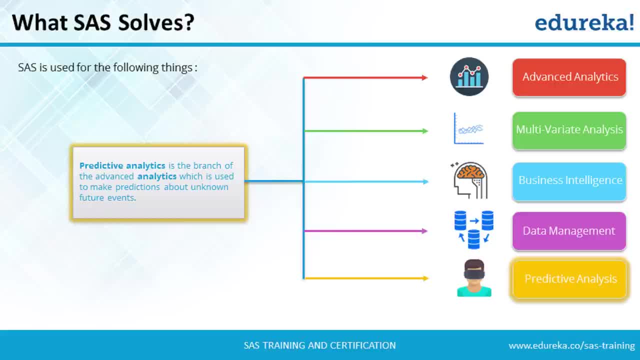 the outcome right, and this actually helps you in better decision making- Right, if you don't know what will happen. so what happens in predictive, predictive analysis- is you rely on the past data. So, based on the past data, you come up with a model, right, So you feed in values that you, or you feed in decisions that you. 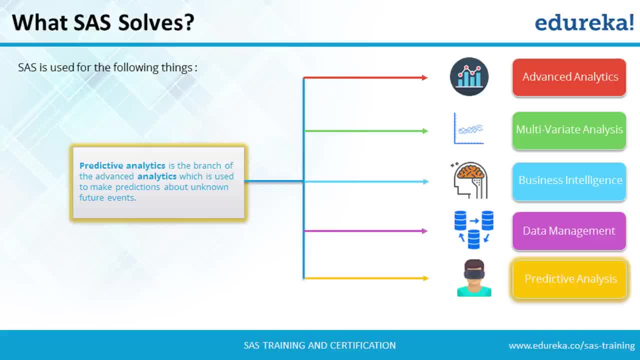 took in the past and then lead to conclusions, right. So, based on these decisions and the conclusions, you come up with a model And on this model, you feed in the new data or the new decisions that you want to make, Before actually making them. you actually feed them. 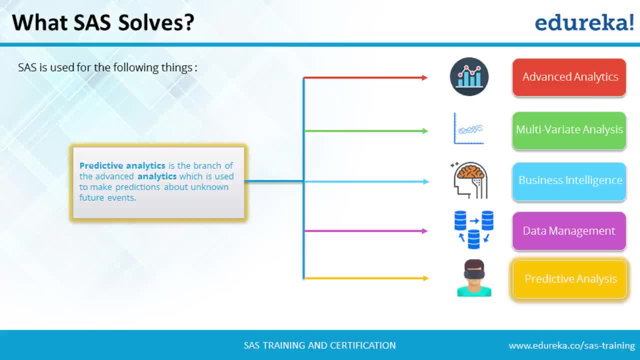 in the model, and this model then predicts a conclusion: what will happen, right, Based on the past trends. So this kind of analysis is called predictive analysis, and SAS can do that for you as well. right? So these are the things that SAS can actually handle Moving. 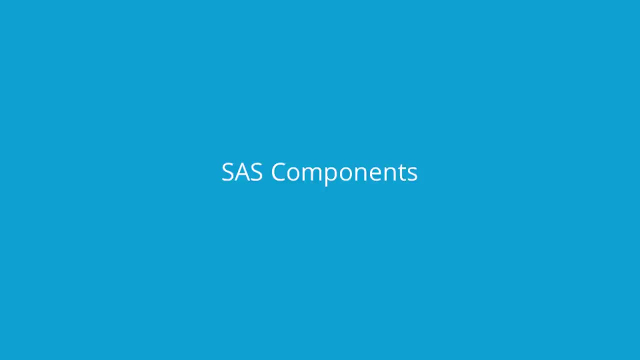 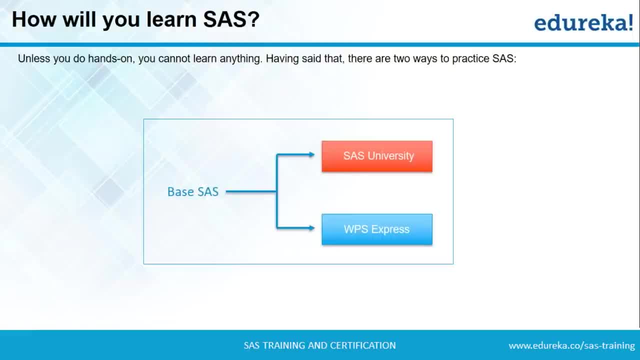 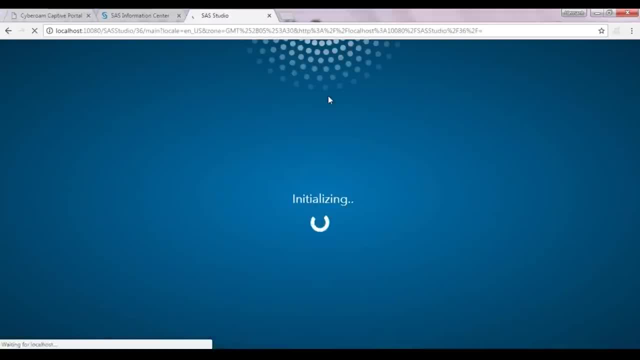 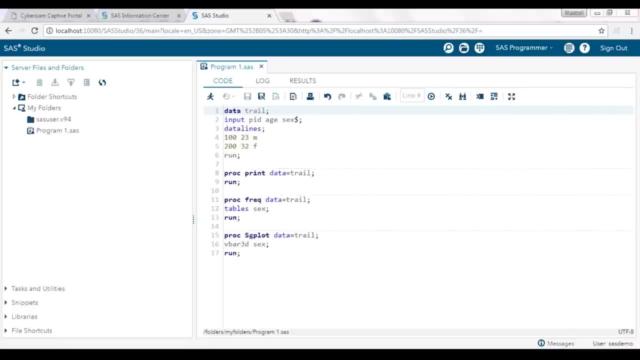 things right, But then all these things cannot be integrated into one component. So SAS can do a lot of things right, But then all these things cannot be integrated into one component. It is initializing now, Alright guys, so this is it right? 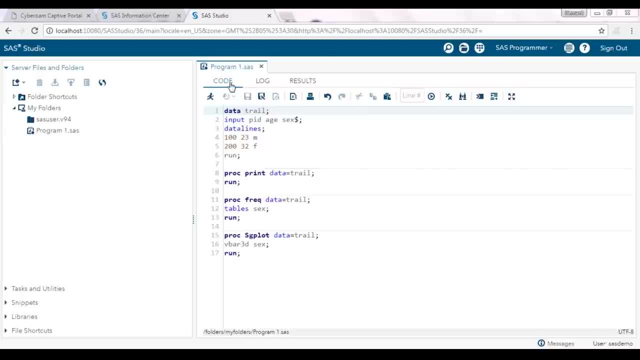 So this is the SAS Studio. You have three things over here: You have the code, you have the log and then you have the results. right. So in the code part you actually give your code, In the log part you get any errors that you'll be getting, and in the results part you'll. 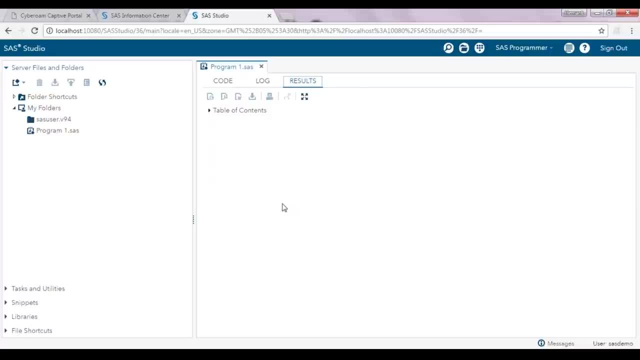 actually be getting the graphs or the tables that you have actually coded the application for right. So this is how your SAS Studio looks like. On the left side you can see that you will have some files and folders. wherever you are trying to store your data sets, wherever you're trying to store your code, all will be listed. 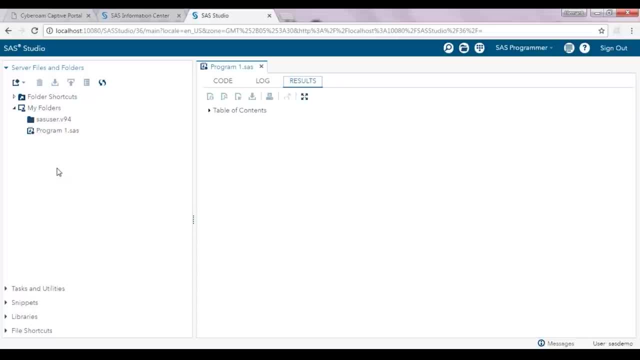 over here, Alright. so, guys, this is how your SAS Studio will actually look like. There's nothing much to it. You have code wherein you'll be coding it, the log and the log. These are the results. Now, whenever you'll be trying to implement or whenever you're trying to execute your 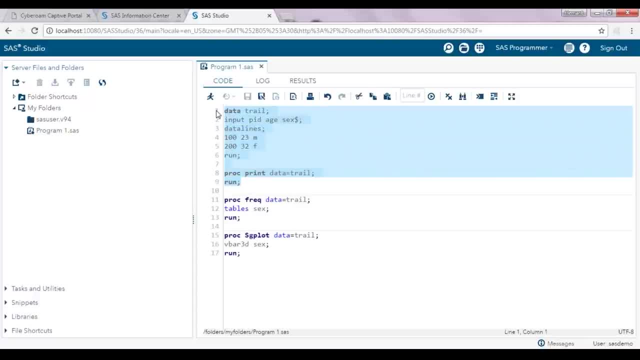 code. what you'll be doing is you'll be selecting that part of the code and clicking here which is run, right, So you click on run and then it will run that particular set for you. So don't worry, all of this is exactly the same in WPS as well. 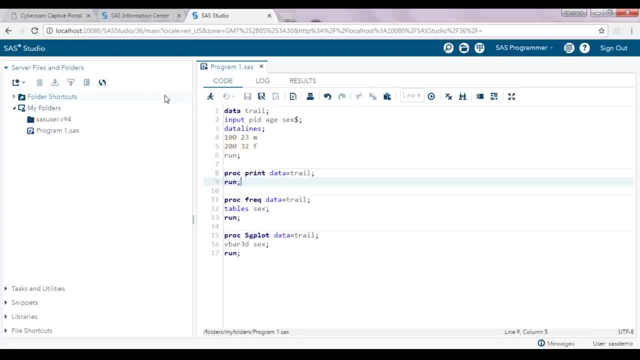 There's no difference, It's just over there. you'll have a different icon for running, So there is nothing that you won't be understanding Over there. Alright, so this is how the SAS Studio actually looks like, guys, so I'm closing it now. 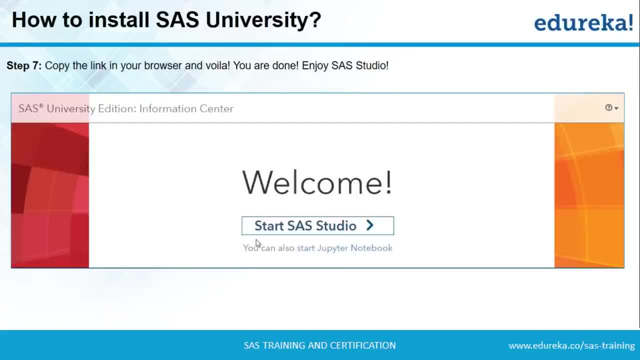 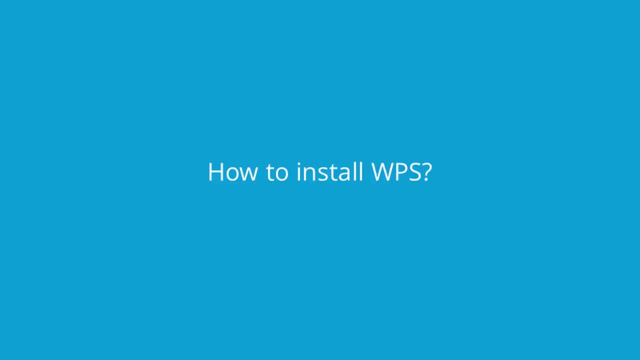 Let's continue with our session. Alright, so this is how you can actually install SAS University. Moving on, guys, I am using WPS, so I don't think you guys should have the need to use WPS, but if you do, this is how you install it. 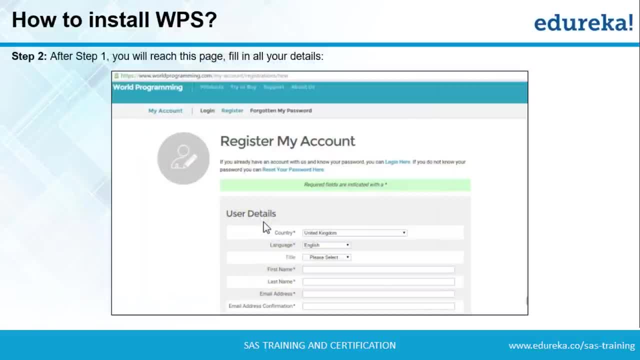 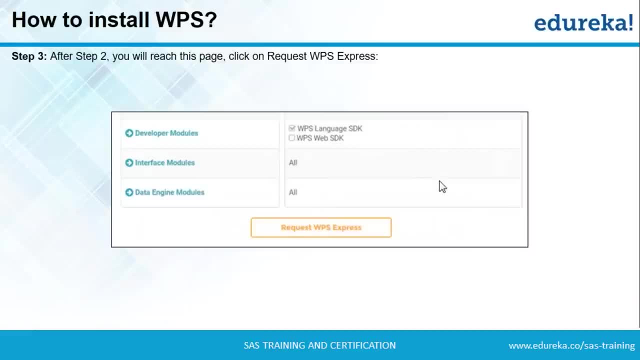 You go to this link and you will see the screen right And then, If you just click on install, you will be prompted with the screen. you'll have to register an account and then you have to request for that particular software. The software name is WPS Express. 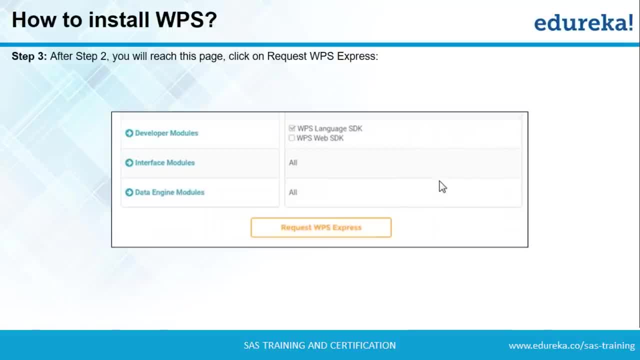 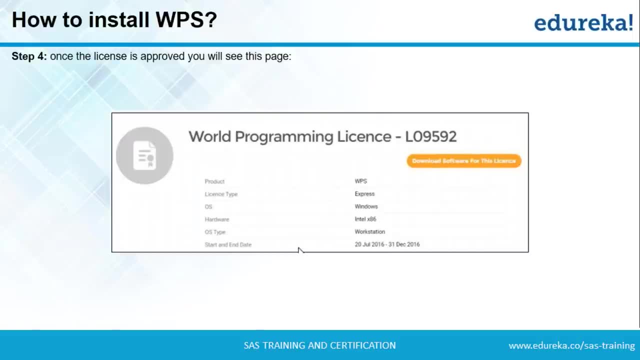 It is free, right, So you can install this free software and then move on to the license. So it will give you a license and then, once the license is actually, it will take around five minutes for it to be approved, or somewhere it will say it will take around one day. it. 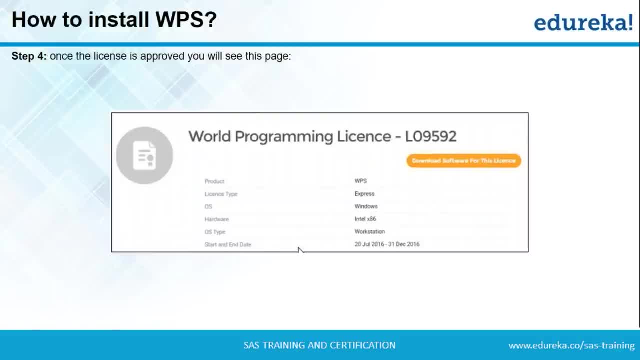 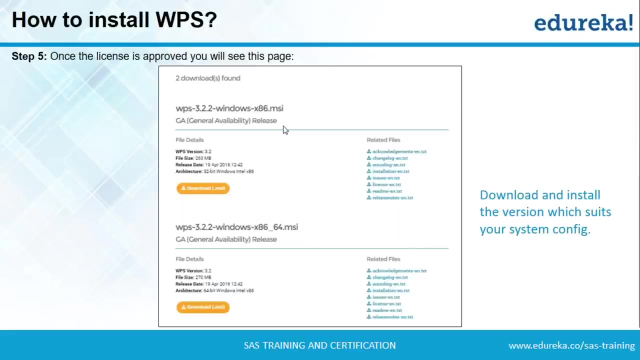 might take, but for me it took five minutes. So you can wait for like five minutes and your license will be approved, And then you can click here. that is download software for this license, right? So once you click here, the installation will actually begin and you will be prompted with: 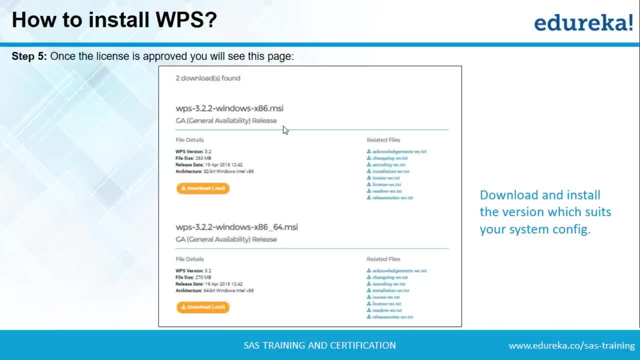 this screen next, And then, according to your architecture, if it's a 32-bit, you will be going with x86, and if it's a 64-bit, you will actually be going for 64-bit. So that's it. 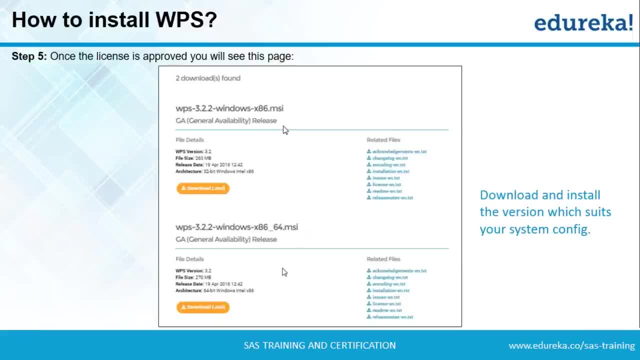 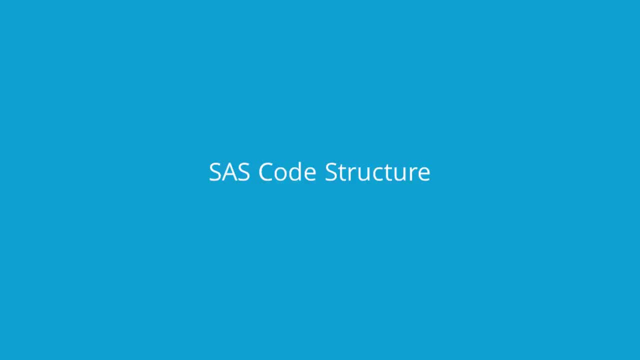 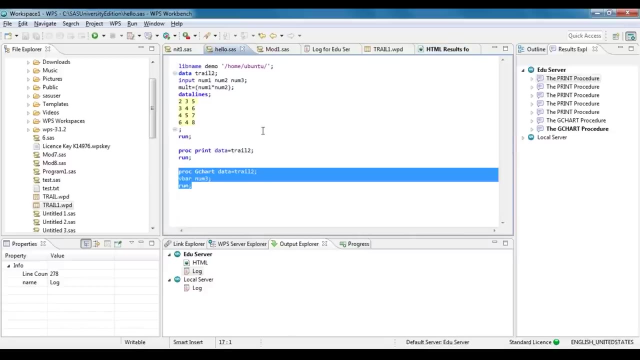 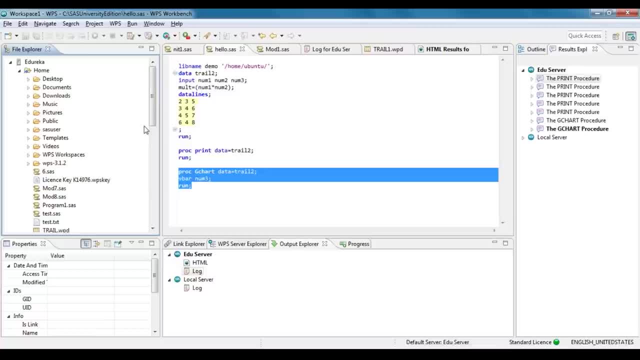 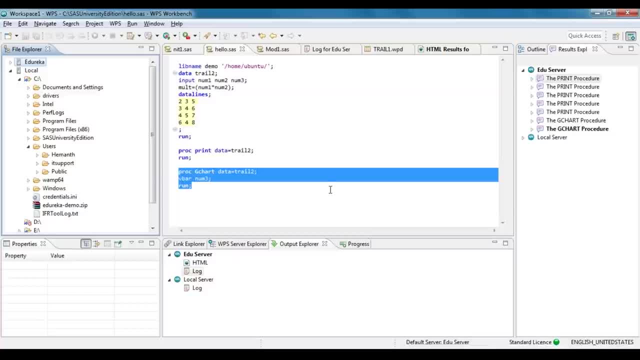 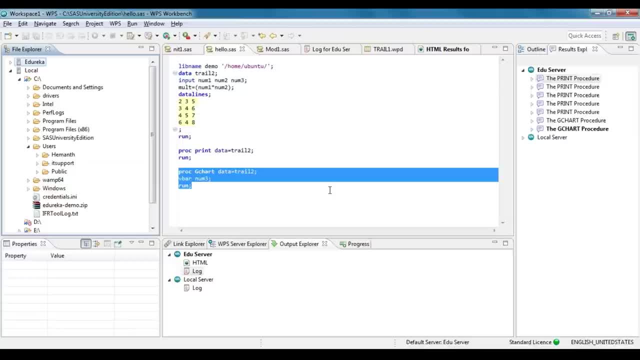 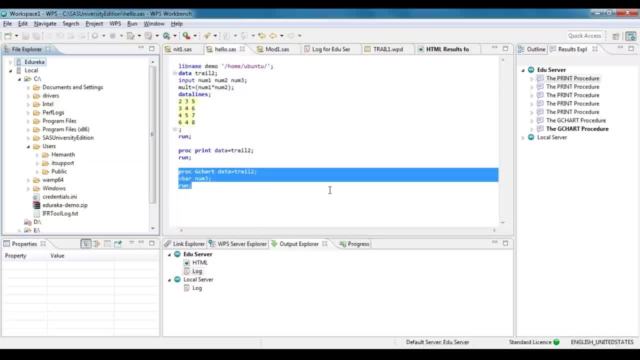 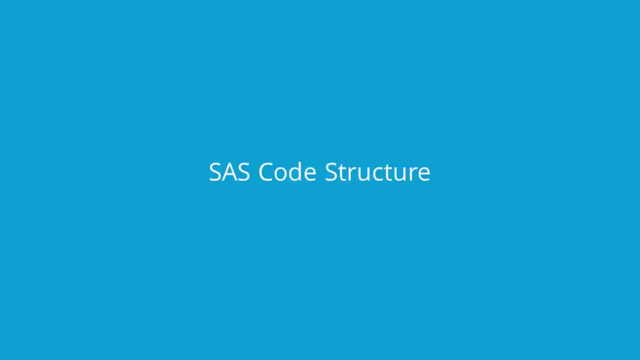 using this licensed version of SAS. But for learning we can use WPS or SAS University, But once you enter the commercial business, you actually have to use the licensed product, Alright. so, having said that, let's move ahead. Now. let's understand the code structure of SAS. So we have now learned how we can. 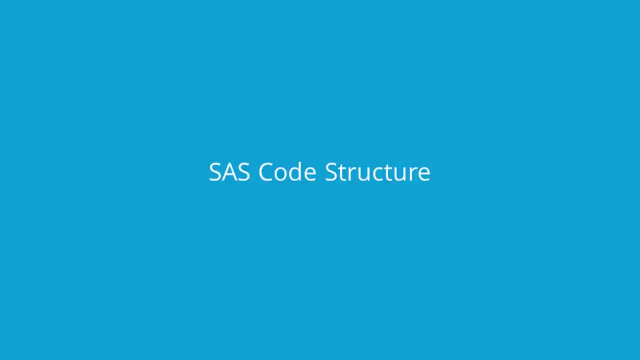 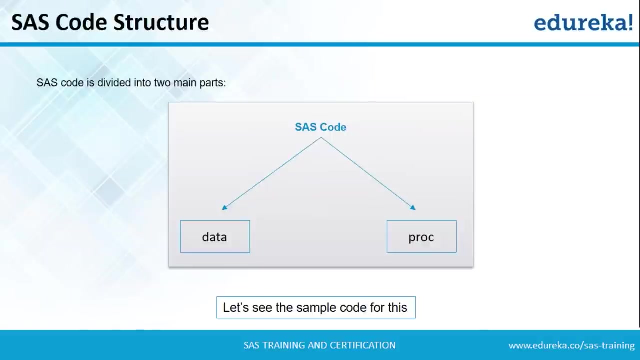 install the SAS software, the relevant software, that is, WPS or SAS University. Now let's start with the coding guys. Let's see how SAS is actually programmed, or how is it structured, right? So basically, the SAS code has two kind of blocks. One is called the data block and the other is 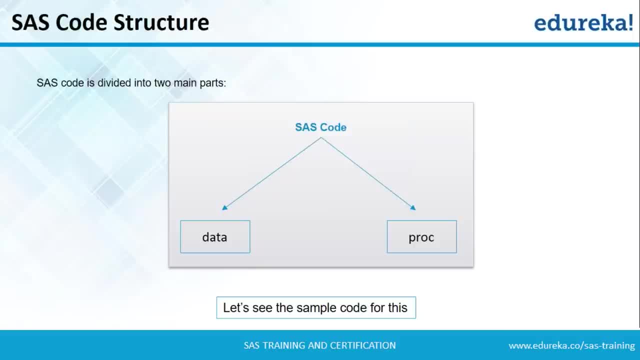 called the procedure block or the proc block, right, So the data block is basically for defining the data set, for performing operations on the data set, and procedure is actually like a function, So it executes, it deals with the execution part of a data set, It deals with the statistics or whatever operations. 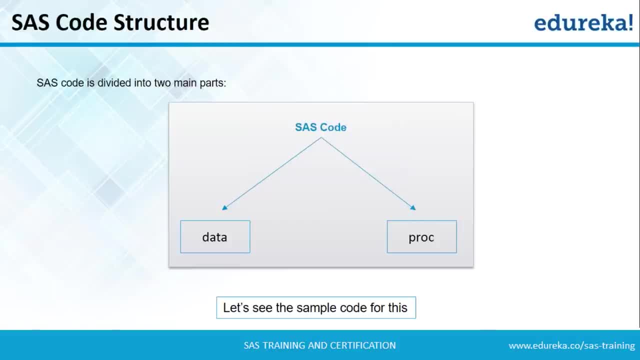 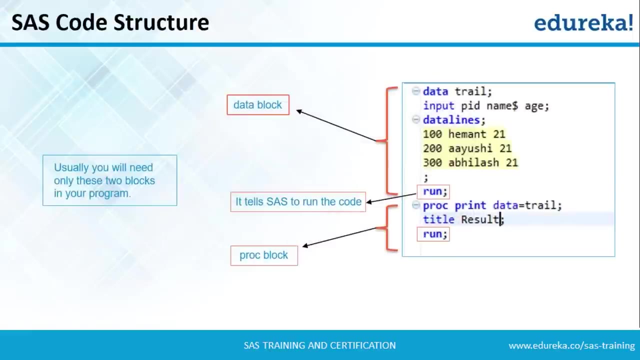 that you want to implement that can be included in the procedure part. So, whatever output that you are seeing, that output is actually coming from the procedure part of your program, right? So, having said that, let's move ahead and see a sample code, right? So this is a sample code, guys. What this code is actually doing is so it is. 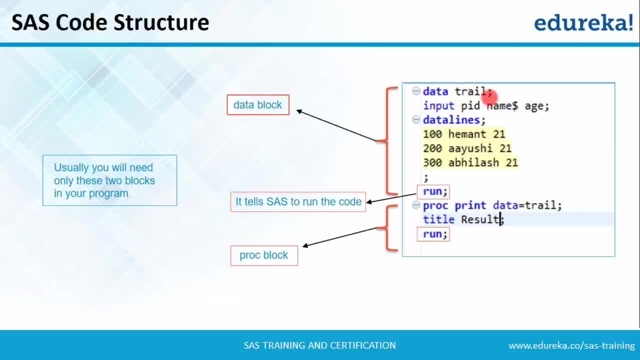 defining a dataset called Trail right, And this dataset will have three columns, which is PID. it'll have name and a lot of age. right Now, PID is nothing but number value. right? Name is a string and whenever you have a string, guys, you have to attach a dollar after it, right? 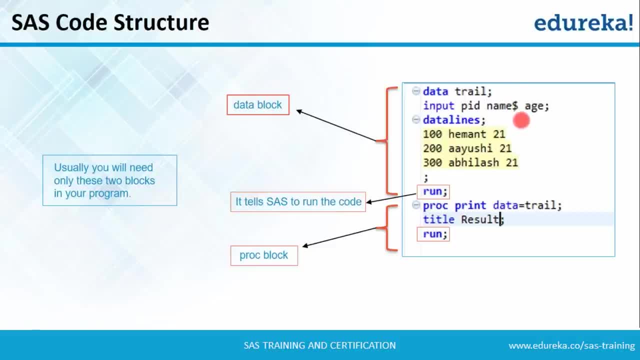 So if you attach a dollar after it, SAS will understand: okay, This is a string. and then you have age, which is again a numeric value, right? So once you have given the input line in the data block, next is you have to give data lines, So you'll be entering. 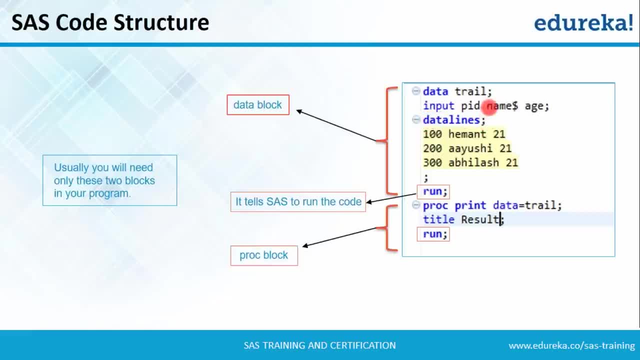 this statement which says data lines, semicolon, and semicolon is very important, guys. after each and every command that you give in SAS, right? So data trail, you see the semicolon. input, PID, name, age, you see the semicolon, and then you enter data line. So data lines means after this command, you'll be. 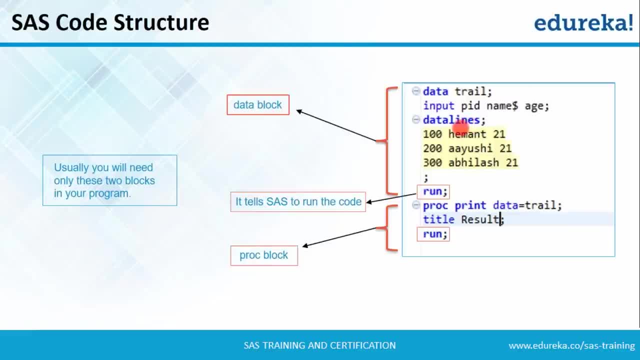 entering whatever records that you want to add to your database, right? So you enter data, lines, semicolon, and after that I've entered three records. So the first record is PID, which is 100. then you have the string which is my name, and then the age, which is could be anything. I'm not saying I'm 21, but then yeah. So 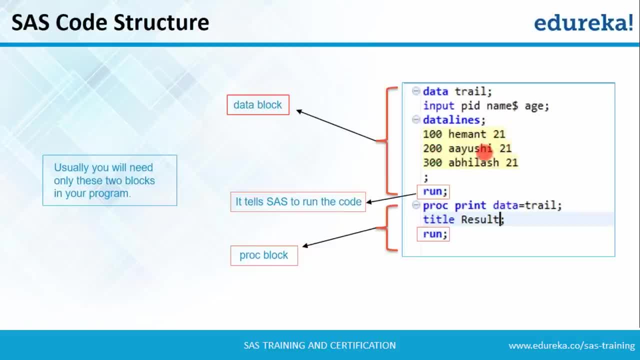 you can enter your age. hit enter, enter the second line. so PID is now 200, the name is Ayush, Age is whatever you feel like, and then you have PID again for the third record. then you have 300, you have the name and the end, the age, right Now after. 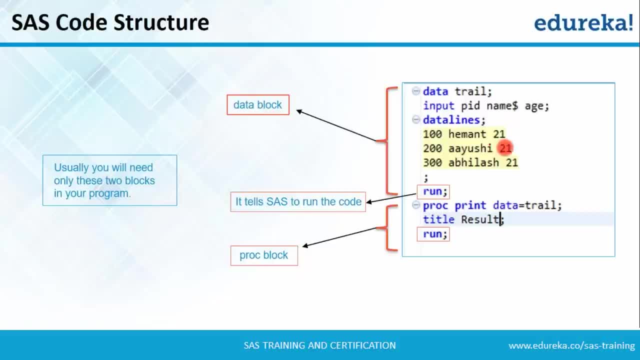 each and every entry that you want to make, you have to hit enter. Remember, guys, there's no semicolon after this, it's a enter, right, You hit enter. you come to the second record. enter the second record, hit enter again. enter the third record, and so. 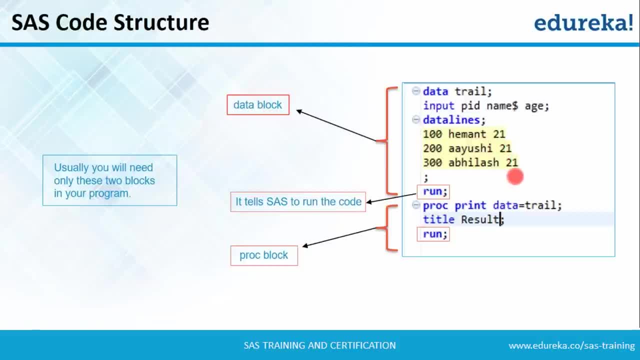 on right. Once you are done with entering records in your data set, you can actually put an end to it by putting a semicolon, So the semicolon marks that you're no more entering any more records. and then, after each block- that is, the data block and the procedure block- you have to enter the run as well. So run. 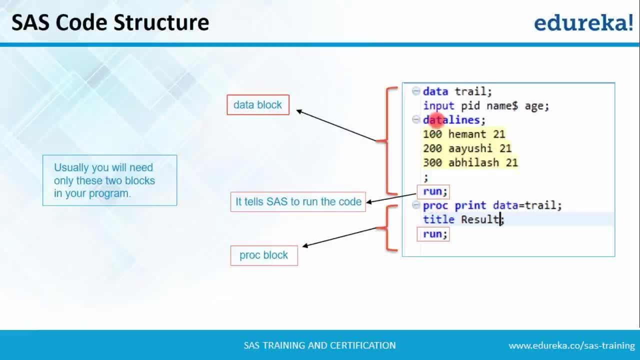 basically tells SAS: okay, so run this particular block now, right. So run is very important and after a semicolon will again come right. So run tells SAS to run the code and then this is the data block, which basically includes the data block Basically includes all the operations related to your data set. and then you 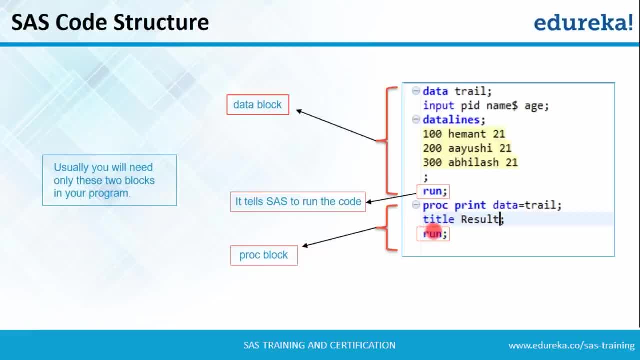 have the procedure block or the proc block, which will contain the output section of your code, right? So in this we are basically printing the data set which we just created, which is called trail, right? So we said PROC and then the print command and then we say: okay, the data set is trail, right. Now the title. 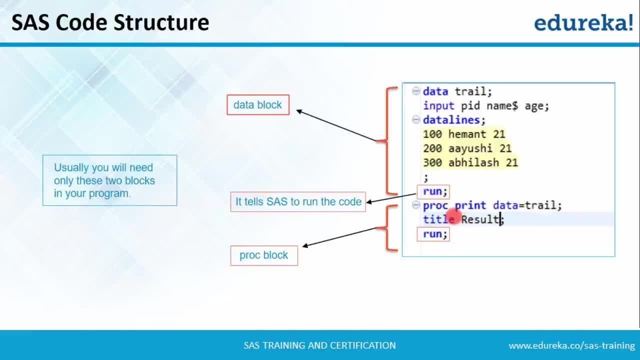 result means the title of that result. whatever we're getting in the result window should be result right. So when we say title result instead of the normal default header which is there, which is the WPS system, you will get result as the title right After that obviously. 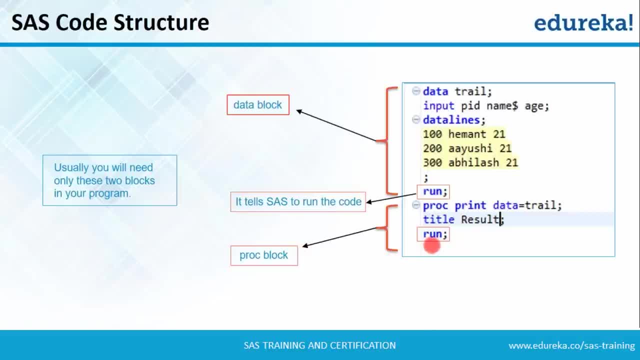 like I said, you have to put run, which basically tells SAS to run this particular block, which is the PROC block, right? So this is basically the structure that is there in SAS. pretty simple, right? There is nothing related to programming in this. This is a 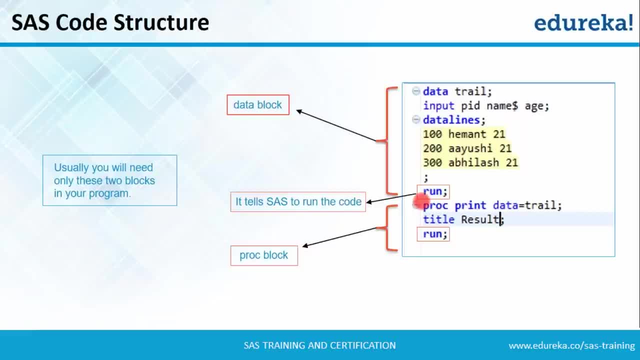 fresh. this is very simple. this is very new for you. So if you follow these guidelines, so basically you have, like I said, there are just two blocks, so there is nothing much to remember as well. alright, Moving on, guys. let's move on to. 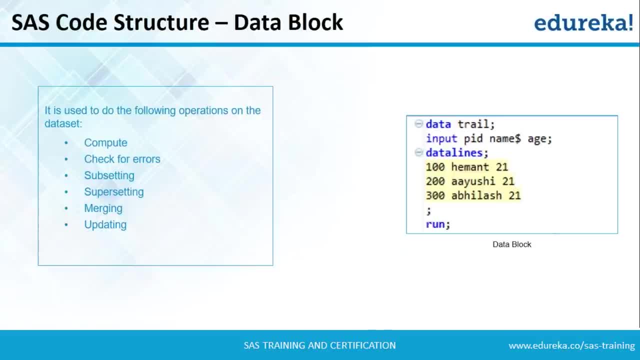 the next slide which talks a little in detail about the data block. So the data block actually can be used to compute data sets right. It can be used to check for errors in the data set. It can be used to subset a data set if you want to. 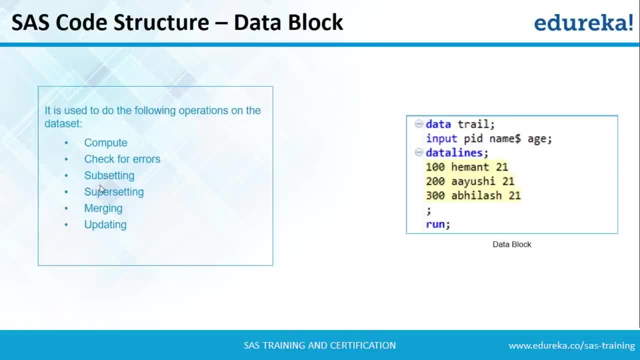 make smaller data set out of a parent data set, you can do that. in the data block It is used to superset a data set. if you want to combine two or three data sets to make a bigger data set, that can be used to do that. It can be used to. 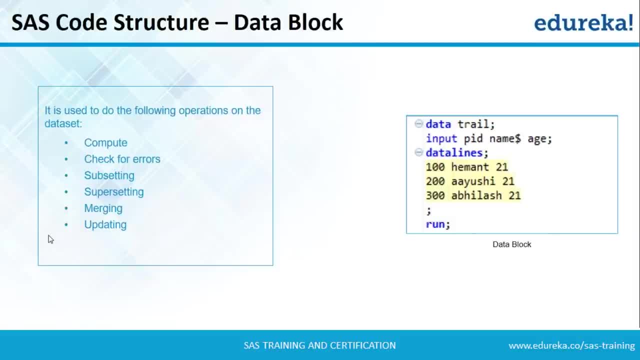 merge data sets, can be used to update data sets, right? So all of these operations can be done in the data block. So, as you would have noticed, all these operations are actually related to your data set And hence they are executed in the data block, right? So, if any nothing in 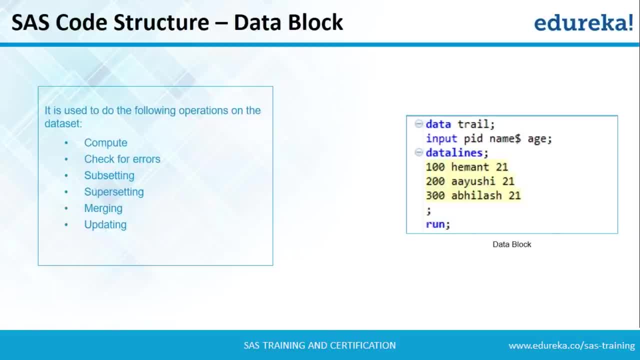 this operation. none of these operations are actually related to the results pain in your SAS Studio, right? So you will see nothing if you execute a data block in your result pane, right? It is only the procedure block which will lead to results in your results pane, right? So this was about the data block, guys. Next, 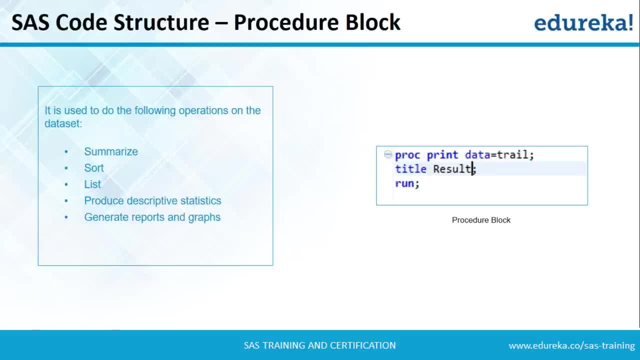 we have the procedure block. So the procedure block is the data block that is used to block. So procedure block is basically used to summarize the results that you're getting. It is used to sort the results that you're getting from the techniques that you're implementing, List the results. It can be also used to produce: 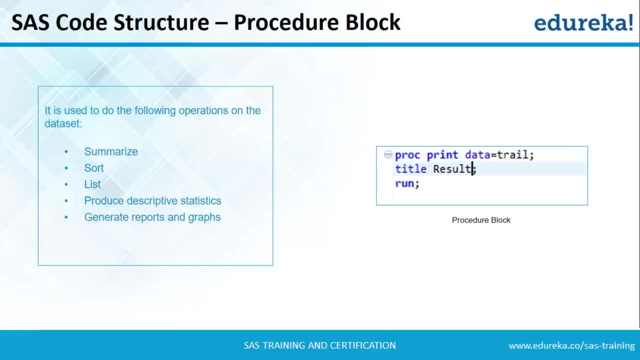 descriptive statistics, as in tables, which will contain probability values and stuff like that, And also it can be used to generate reports and graphs, Right? So if you want to visualize something that also has to be done in the procedure, block Alright. Having said that, guys, so this was the structure of 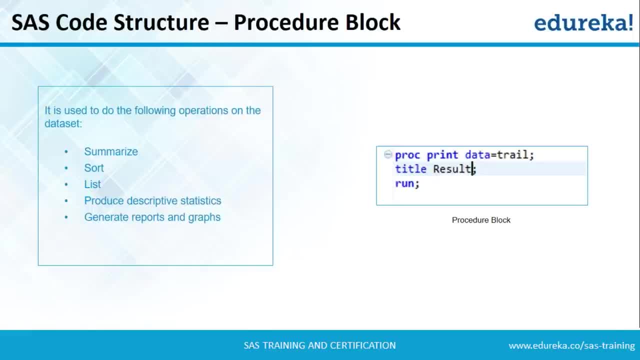 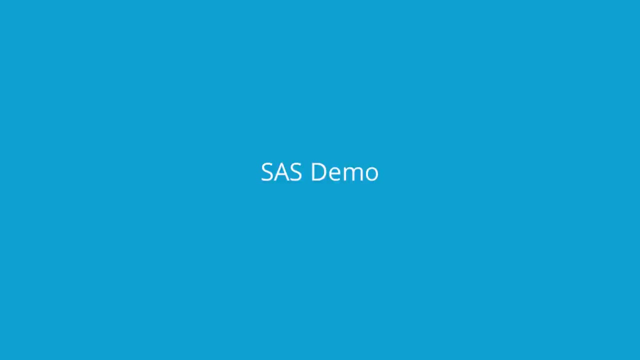 your SAS code. So we now know how to actually install the SAS software. We now know the code structure of SAS. So what are we waiting for? Let's jump on to the demo part. Let's implement a demo in SAS now. Right, So the demo is going to be. 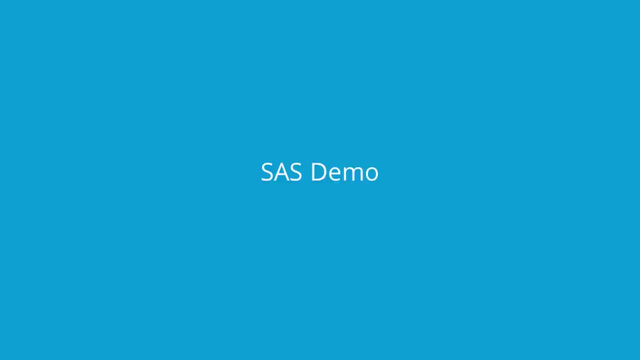 like this. So first of all, let's go to the demo part. Let's go to the demo part. So first I'm going to show you a couple of basic statements in SAS, So basic commands that you can run in SAS, Basic things that you should know as a 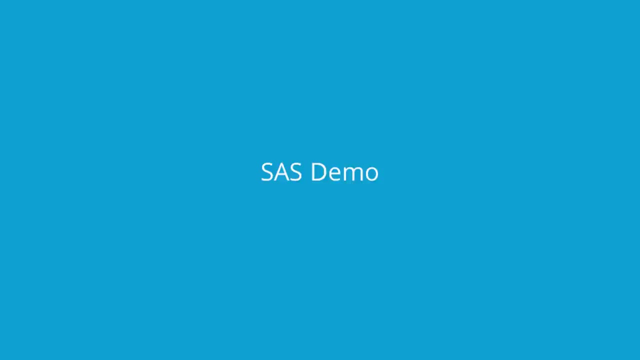 beginner What can be done? Right, Then I'll tell you guys how you can create a data set in SAS. We'll be creating a data set and then we'll be listing that data set in different ways And also we'll see, if we have created a data set, how we can. 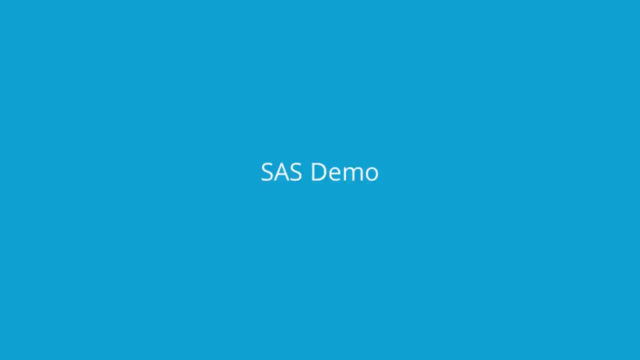 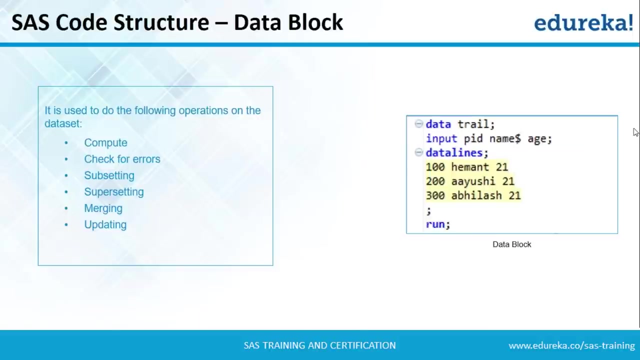 actually save it, Right? So there are basically two kinds of data sets in SAS, right? So if you would come back to the screen, guys, you can see that we created a data set called Trail. right Now. this data set is actually there until you are running that SAS session, The moment you end that. 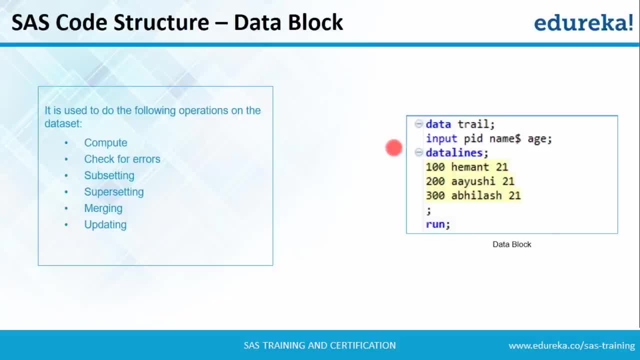 SAS session. this data set will actually go away. It will not be there anymore, Right? So if you have to save your data set, you can do that using the library command that I'll be showing you in the demo, right, So, using that. 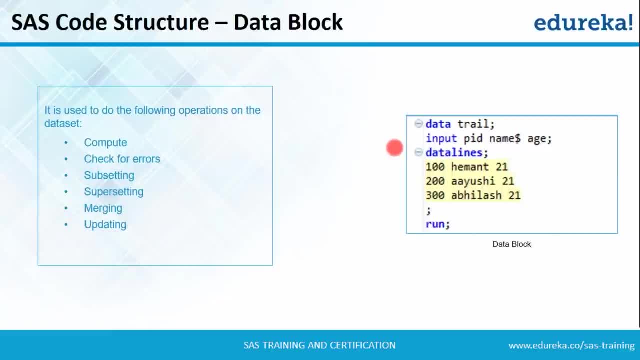 that command, then this data set actually becomes a physical file and gets stored in your file system, right? So this kind of data set is called a permanent data set. After this you have the temporary data sets which are there till the session is running. in your SaaS, For example, this trail data set as of now. 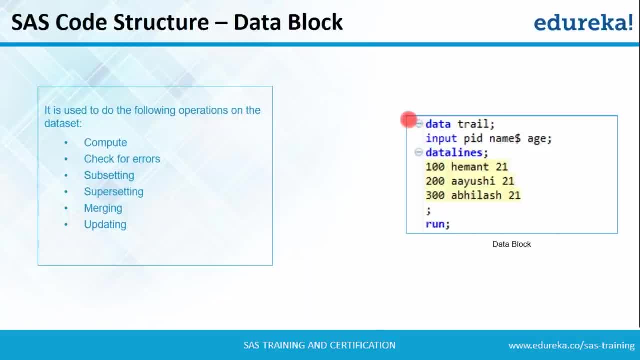 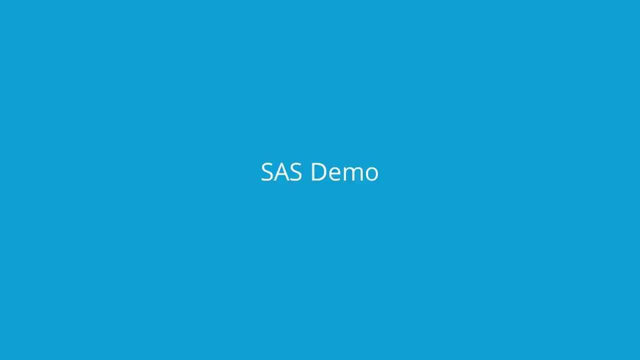 ever since we have not executed the library statement. this data set is actually called temporary, because the moment I'll end my SaaS session, this trail data set will also get evaporated, will not be there in the system anymore. alright, So this is what we'll be learning in the demo part. that is how to. 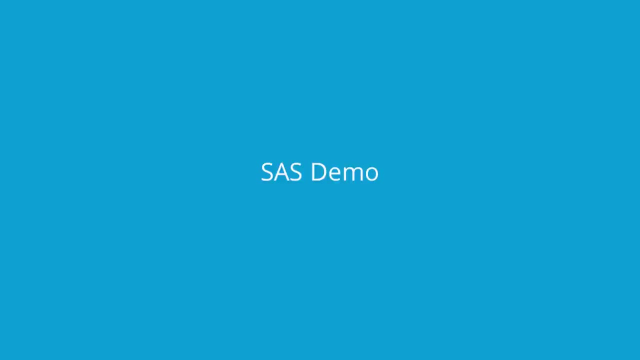 create permanent data sets. We'll also be creating a data set and then we'll see how we can actually update that data set right? So when you create a data set, you're actually creating a SaaS table. Now we'll see how we can actually apply. 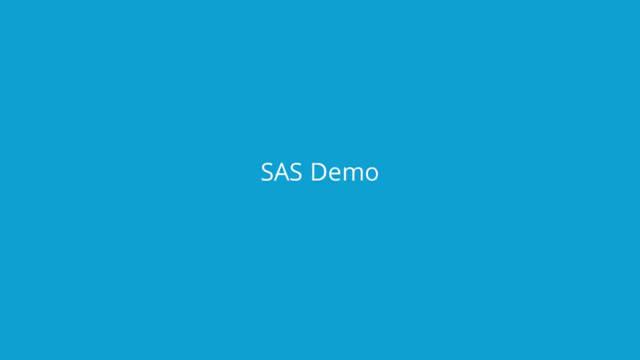 operations in table. So if the fourth or fifth variable is actually dependent on one of the variables in the table, we'll see how we can update or how we can create a new data set using the older data sets and adding a new column in it which is actually dependent on the older variables, right? 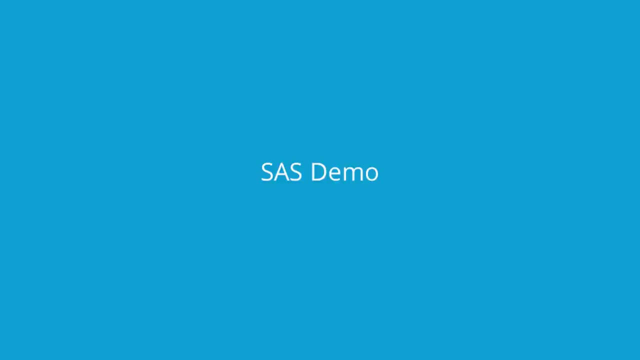 Sounds a little more complex, but don't worry, guys, we'll be going step by step and everything will be clear to you in the next few minutes that we'll be doing the demo for. alright. So let's go to the WPS system. alright, guys. so this is my 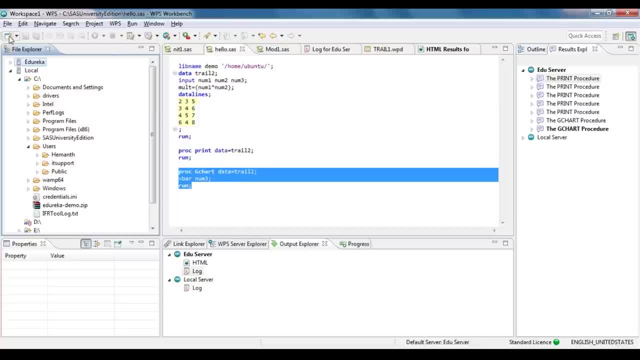 WPS system. So, as of now, me create a new program. We will click on untitled program. Alright, so first of all, like I said, you have to enter the two blocks. So we have the data block. So let's create a data block first. We are creating a data set called trail and 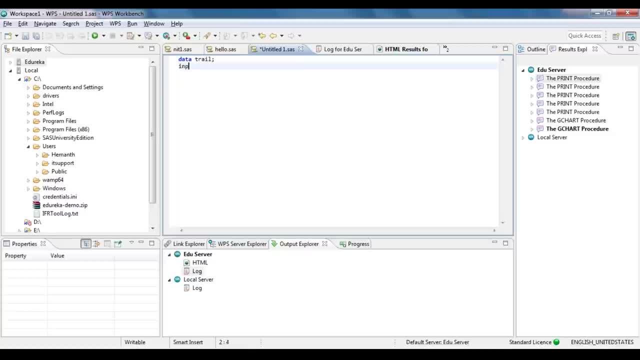 then we want three columns in it Say we want input, we'll enter input. and then let's say we are entering values such as the employee number, the name of the employee and then the salary of the employee. Alright, now, like I said, the 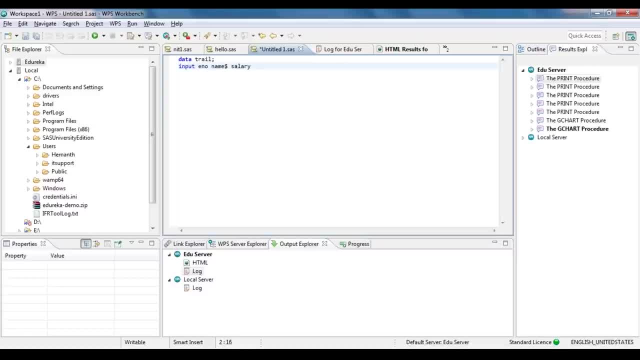 name is string, so you have to attach a dollar after it, and with every statement ending, you have to add a semicolon. Alright, so we're done with the semicolon, Let's go ahead Now. we have created a data set called trail. We have 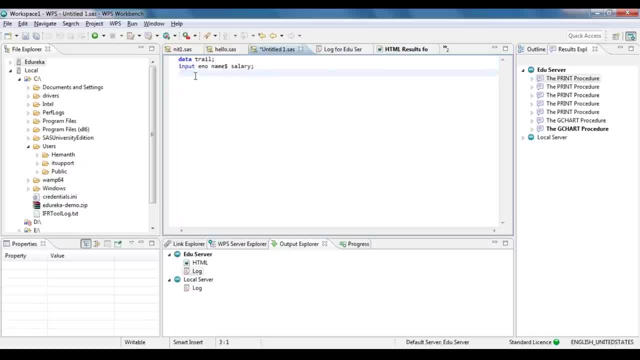 specified that these are the three columns that will be there. Now let's enter the values. So for entering the values, you actually have to write the data line statement, add a semicolon after that and then you'll notice that whatever values that you'll be entering now will come in yellow. That means that 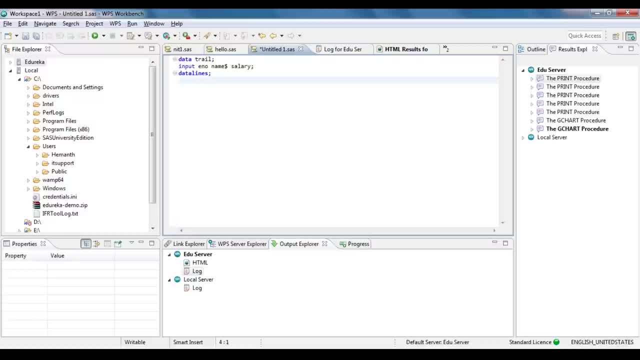 you're actually entering the records that you want to be there in your data set, Right? so first the employee number. so let's give it one right, and whenever you have to move on to the second column, you just enter a space and that is it, Right? so now the second column is name. so let me. 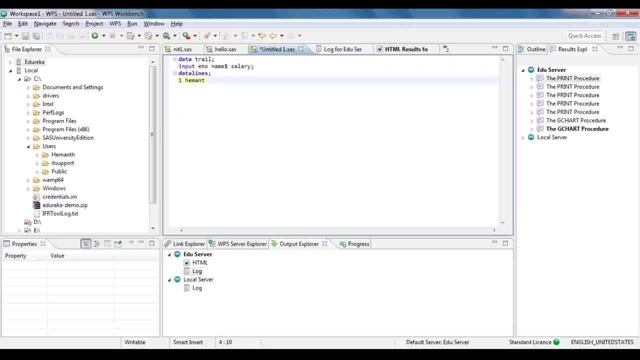 enter my name, which is Hemant. Give one more space. now it talks about the salary, so let me enter my salary, which is okay. let me enter a pseudo salary, which is ten thousand bucks. Alright, the next line will be the employee number. right, so let me enter one more record. Employee number is two. name is say: 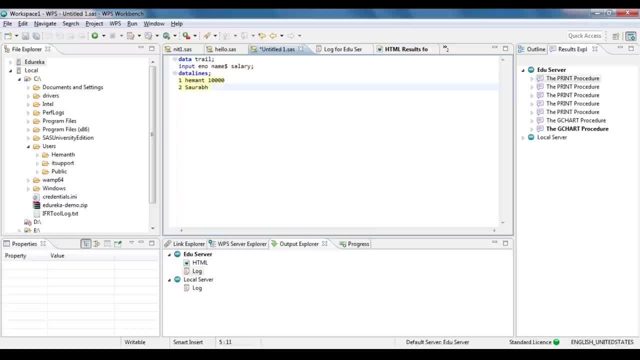 Saurabh right, and the salary is fifteen thousand. Okay, so next employee is, say, Bibik, and the salary is twenty thousand. Alright, so okay, three records we have entered. Now, to mark the end of the entering of your records, you will say: 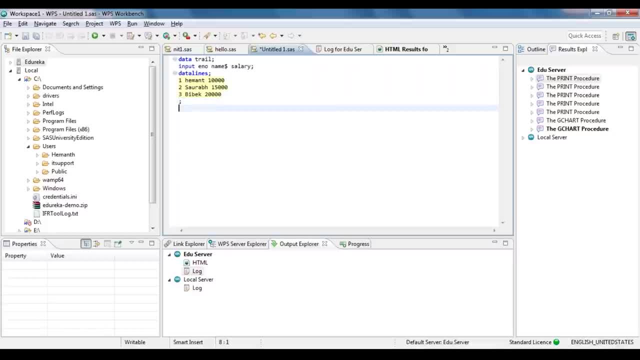 semicolon and hit enter, So done. you won't have the yellow lines now, and then you're done with the data set. You will type run and a semicolon, So this is how your data set will be created. In the next line, let's print the data set. so we'll be entering the proc statement, Alright, so. 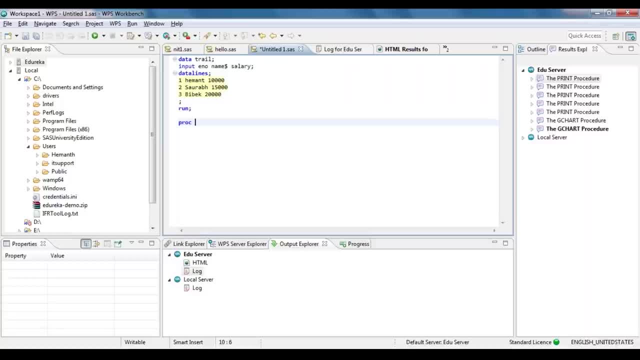 proc. so this is basically means that this is the proc block and then the function that we want to implement. so you want the print function to be implemented, and then I want the data set to be trail, right? so I'll enter the data set as trail, followed by a semicolon Enter. After that, nothing else is needed. 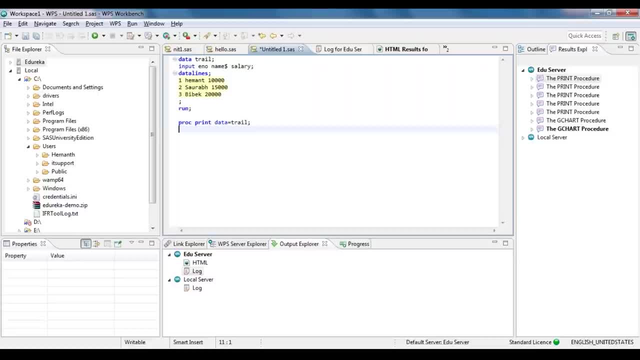 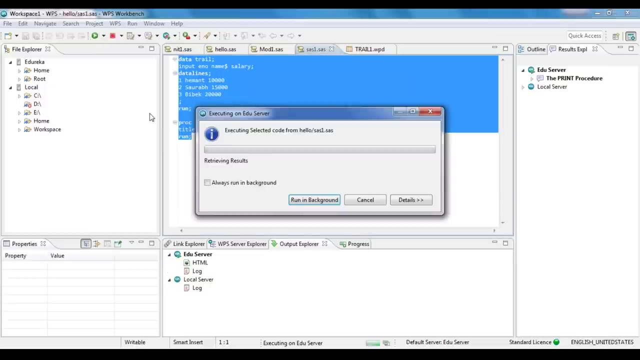 I can give a title right, so the title could be say: my first result right and semicolon followed by run Cool, Alright, guys, so this is our code. let's run it now. Let's select it and click on run right, so it is running my code on Edureka server. 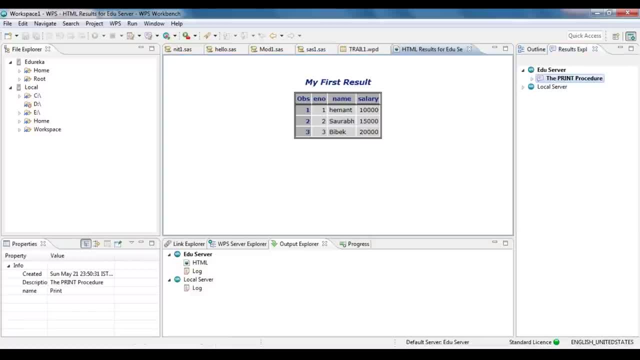 And, as you can see, it has given me a result Alright. so, as you can see, it has printed the results that I have entered. Let me quickly show you. So, SAS 1: I've entered Haman, Saurabh and Bebek and the salaries and the employee number and as 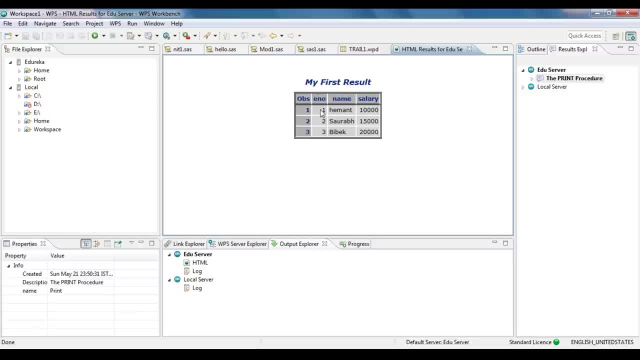 you can see, the title is my first result and the entries are Haman, Saurabh and Bebek, along with their salaries, right. So congratulations on your first program, guys. So you have successfully started coding in SAS. Alright, give me a moment, let's. 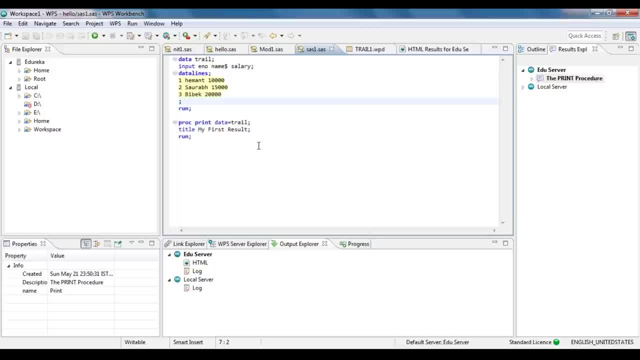 move on to the second part of now. So we have implemented the code for printing a data set right Now. like I said, if you want to actually save a data set on your machine, the way you will do that is like this, right? So you write libname. 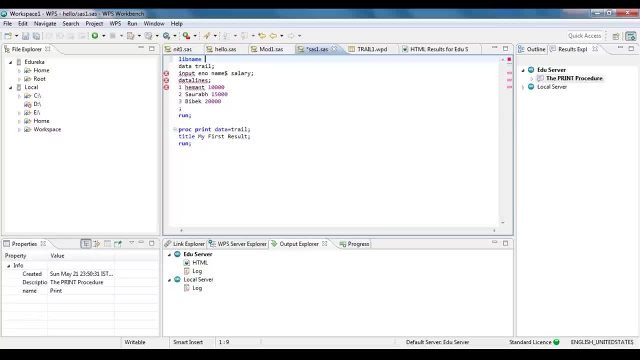 which is libname, right. and then you'll be specifying the library name, so let the library name be demo, alright. and then you have to specify the path. So the path is actually of my Eureka server, so I have to specify the Ubuntu path, so let 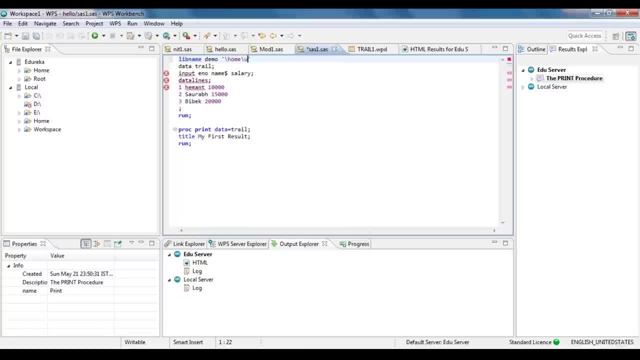 me do that. So it is home slash Ubuntu and followed by a semicolon. right After that in the data statement you actually have to specify demo dot trail. so this is where my data set will be saved right, and let's give it trail 4, because I 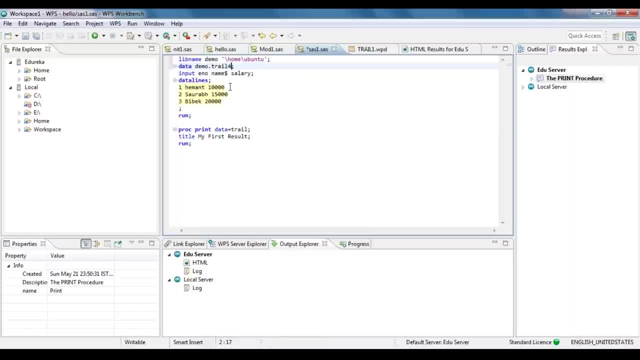 already have a file called trail in my system. Alright, guys, so now what will happen is first it will set the paths of demo as this right, and then I specify that the data should be saved in trail 4.. Alright, so this result that I got is: 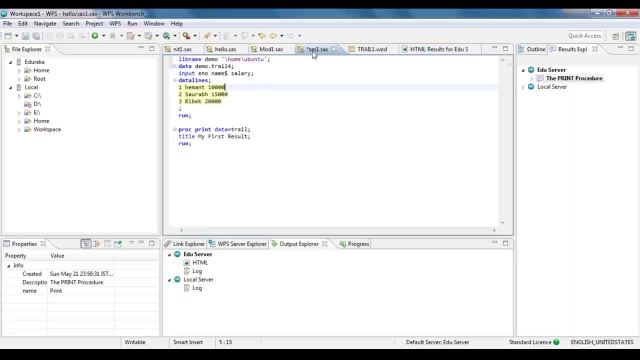 from a temporary data set, but I'm trying to make that data set permanent, Alright, so let me do that. I'll show you the results. I'll show you the home directory as of now for my server. right, So there is no file called trail 4 over here. right, So there's nothing called trail 4.. So now 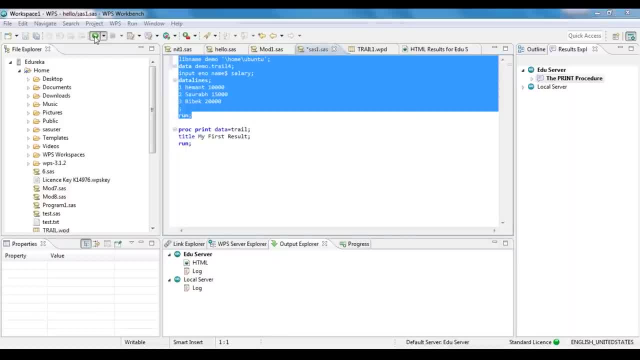 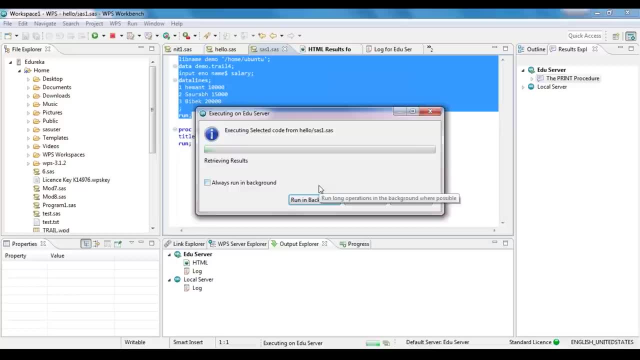 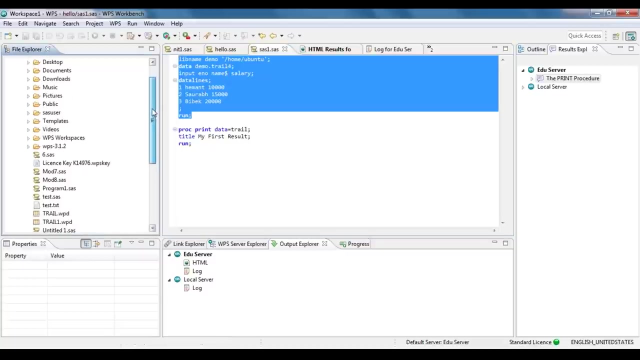 let me run the data path. So I click on data, click on OK, Alright, so, as you can see, the command executed successfully. So I wanted something called trail 4, right? So let's check if there's a folder file here called trail 4.. It is not there yet, Let me refresh it. 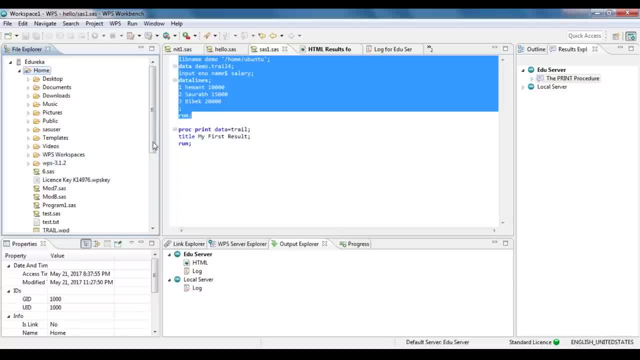 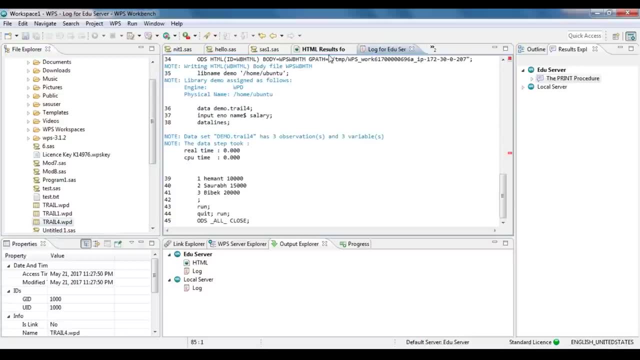 right. So the moment I refresh it I'll see a file called trail 4 over here. So, as you can see the file called trail 4 here now, right. So my data set was this right: It should have Haman, Saurabh and Vivek. Let me check what this data set has. 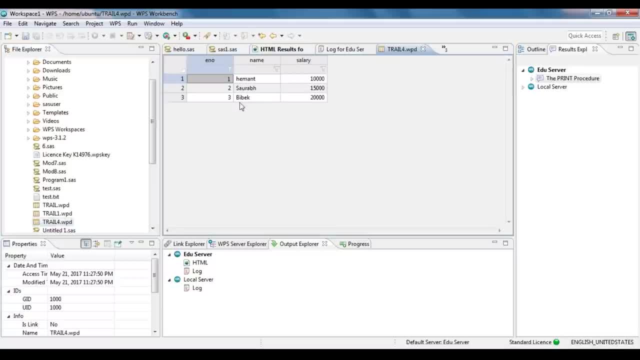 Alright, so this is what my data set has: Haman, Saurabh and Vivek, 10,000,, 15,000 and 20,000, and this is it, guys. So now your data set is actually permanent. Now let us create one. 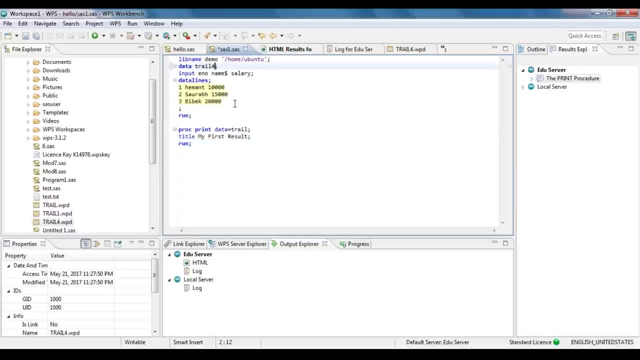 more data set, right, Let us create a temporary data set called trail 5, right? and then we want it to be a copy of trail 4, right? So we'll say set trail 4.. So, which is in demo? right? So we'll specify demotrail4 and hit, followed by a. 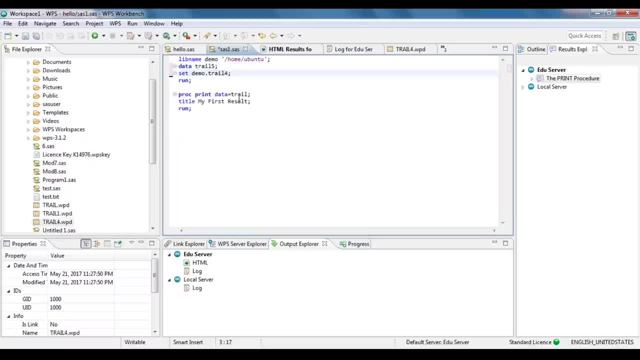 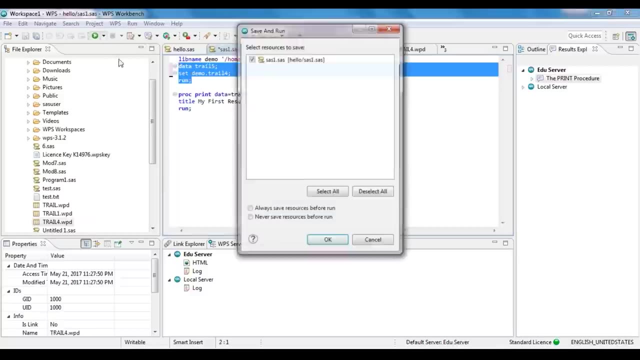 semicolon, right. So now what will happen is it will create a data set called trail 5, which will be an exact copy of trail 4.. For that we'll be using the command called set in the data block, right? So let me run this statement. 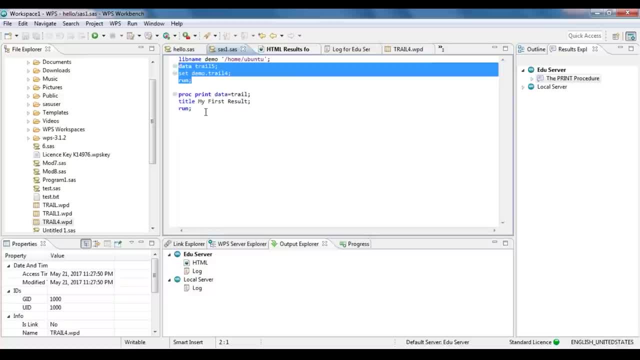 Alright, So my statement executed. Let me print it now. So, data equal to trail 5- my first result from copied data set. Let's try to print this. So I have entered the data to be trail 5, right, and the title is my first result from copied data set. Let's try to run this statement. 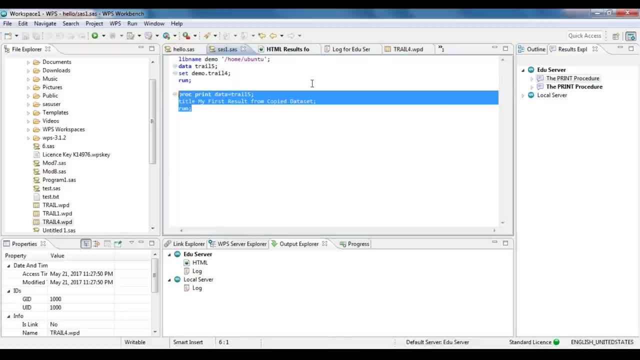 All right, I've got a result, So let's see what a result says. So, as you can see, my first result from copied data set, and then you have these three records which have been successfully been copied from the permanent data set. Alright, guys, So now what I want to do is: I have copied the data set. Now I want to. 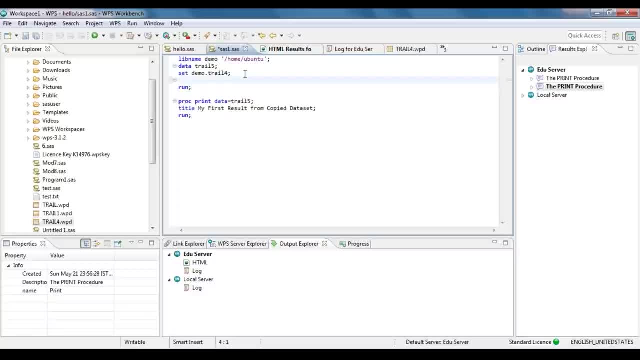 add one more field to it. Let me add one more field to it to it, which is say MUL. right Now, what is MUL? MUL is nothing but the salary multiplied by 2.. Alright, so basically, this column will contain the salary. 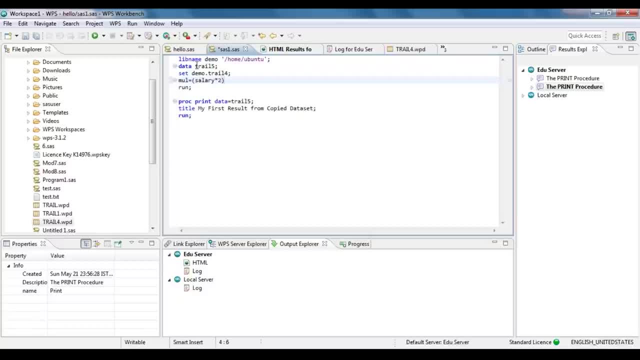 which is multiplied by 2, and I am saving it in trail 5, which is my new data set, alright, and I am taking a previous data set, that is a trail 4.. So, basically, what I'm trying to do here is I'm taking a data set which already exists and I'm 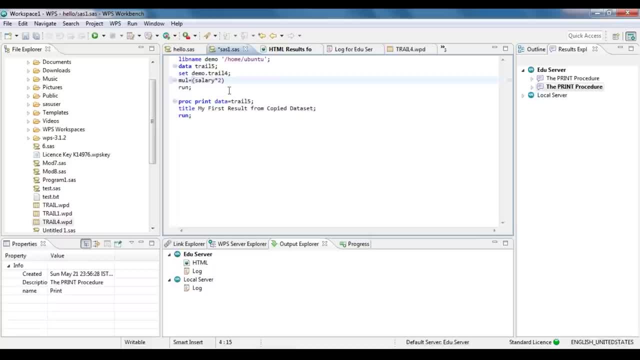 adding one more column to it, which will be actually dependent on the salary column from trail 4, and what I'm doing with that is the dependency is that I'm multiplying it by 2.. Alright, so let's sort of run this whole code. Click on OK. 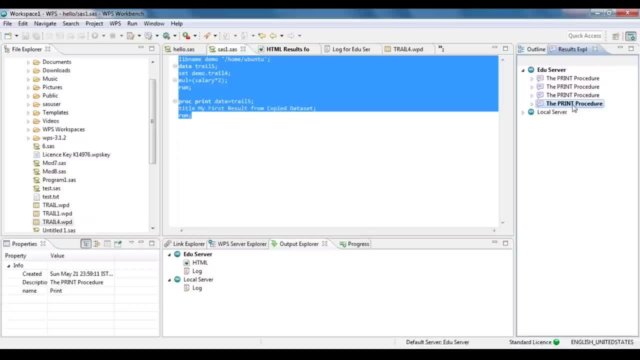 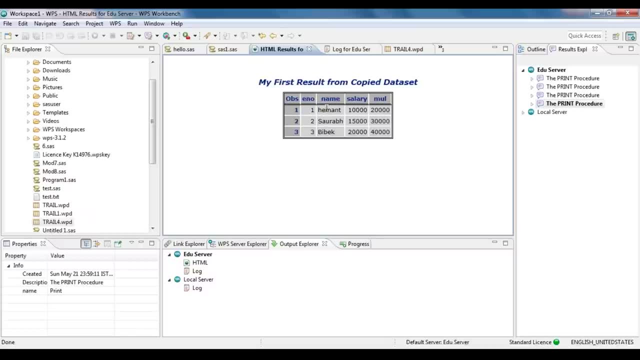 and we are set. Let's check the print command what it has to show us. So, as you can see, we have copied the data values from trail 4 to trail 5 and added one more column, which is MUL, which is nothing but the multiple of salary by 2. 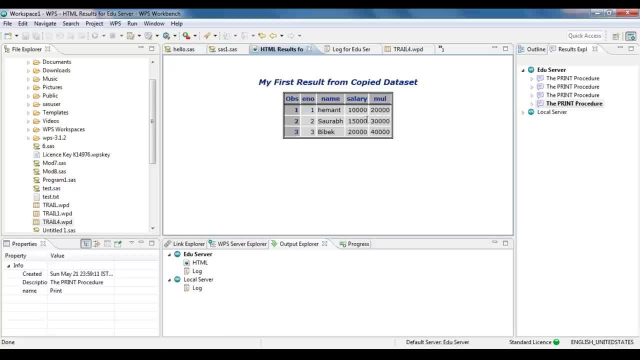 so 10,000 becomes 20,000, 15,000 becomes 30,000 and 20,000 becomes 40,000.. Alright, so we have done this as well, guys. So let's now end this session, but let me give you a little more procedure statement than you can do, which I think. 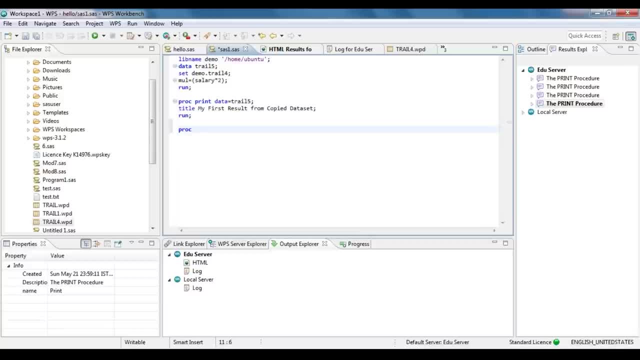 should not be very complex. So let it be procedure, and then I'll say g chart. So g chart is basically used for creating graphs, right, and I want data set to be trail 5 title. okay, let me give it title as my first chart and the next command that I want you guys to see is vbar, right, so I want that. 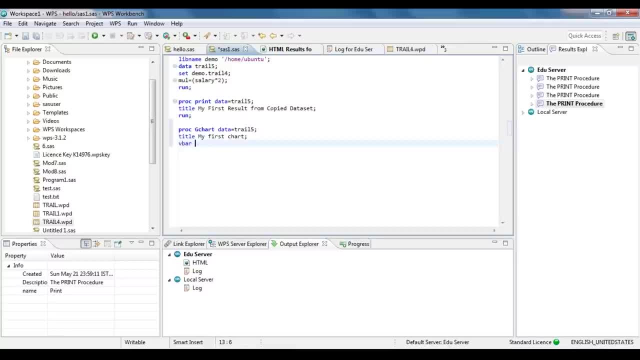 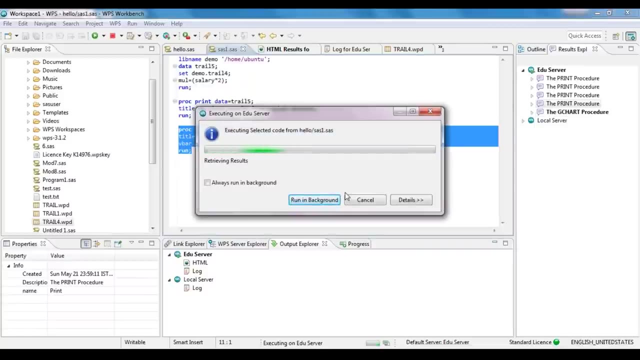 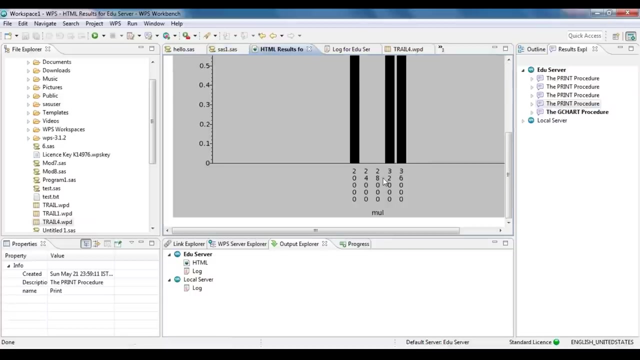 to be on the salary on the column MUL right, and then I'll be closing it off by saying run Alright. so let us try to run this command and see what is the result. Okay, so I've got the result here, alright? so, as you can see, I have implemented the 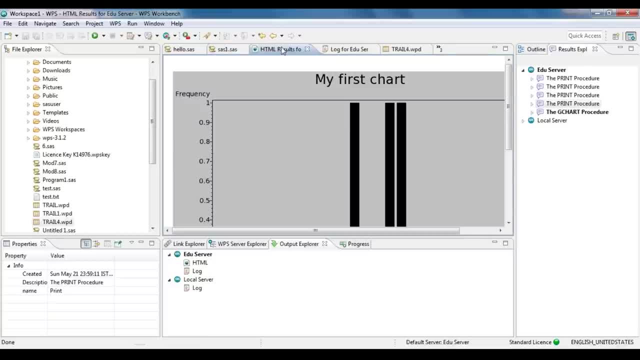 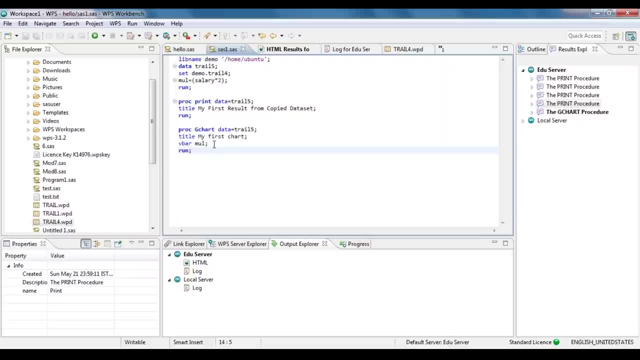 salary on. I've actually created this, so this graph doesn't mean anything, guys, but this is how you can create this chart, right. so, basically, what I'm trying to show you is how to create a chart right. so if you have a frequency table, or if you create a data set and you want to have a chart for the 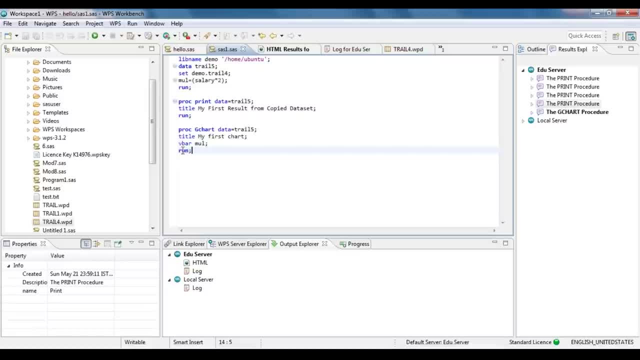 frequency for every record that you have in that data set. So you can, you do that using this particular command, which is so you write proc. that is procedure. then the g chart, which is basically the command for global charts, and then you'll be specifying a data set which is trail 5, and then the title. 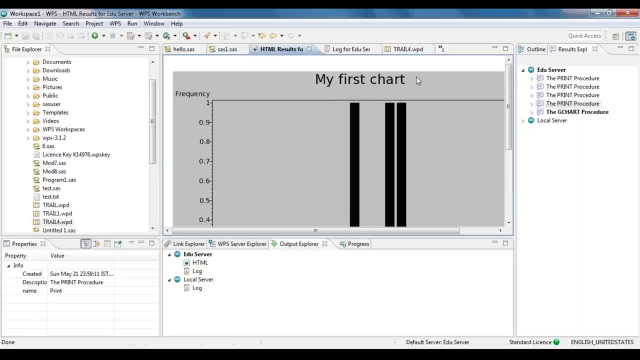 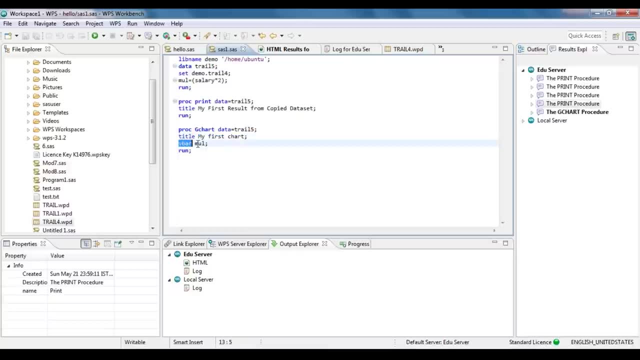 which will say my first chart. so, as you can see here, it says my first chart, right, and then you'll be specifying the column it should be applied on. so you want the vertical bar to be on the MUL column in the data set, and then you are. 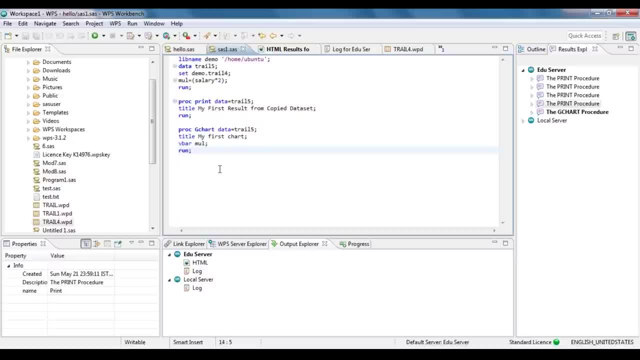 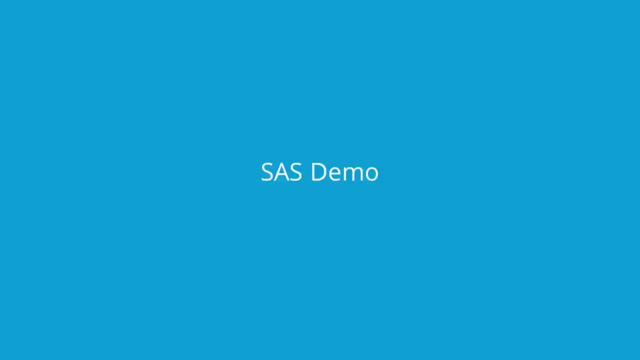 basically running that command. Alright, guys, so this is what SAS is in a gist. so the idea that I want you guys to take from this demo is: SAS is all not that difficult to write. SAS is very simple, it is very easy to understand. right, and whatever you have learned today: data block and the procedure block. this is it. 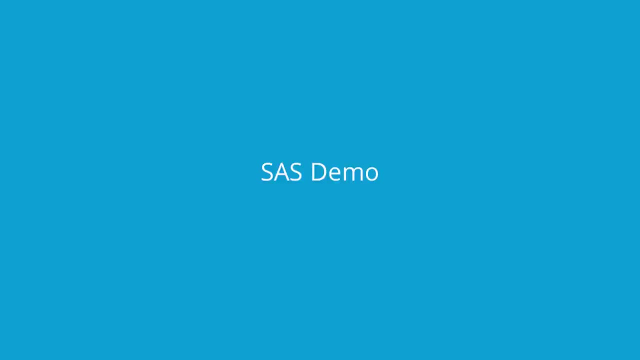 guys, there's nothing more to it. you'll be just typing in more commands and you'll be implementing different procedures. you can apply different algorithms in your process, The block, which is logistical algorithm or sentiment analysis. you can do anything in SAS, right, but whatever you will be doing, whatever functions that. 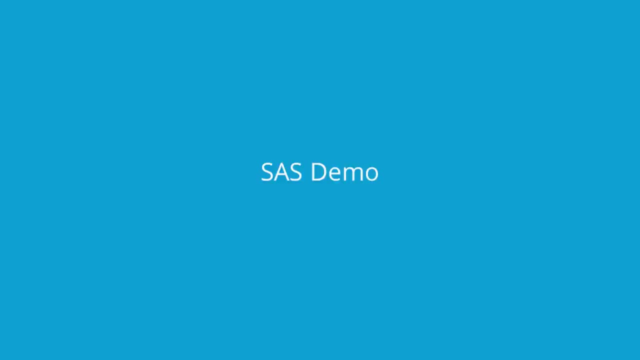 you'll be applying. you'll be applying in the procedure block and you'll see in the upcoming sessions. this is the structure that we'll be following. I've shown you some of the commands, some of the basic commands which are there in SAS right and based on that also, I have prepared some assignments. so I want you 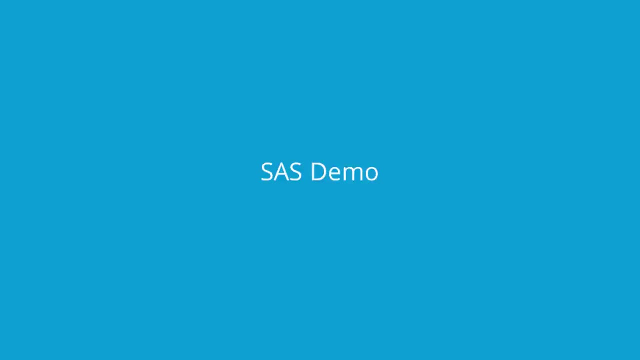 guys to go through those assignments and absolutely guys to be very careful with that right. So this is the first thing that I want you guys to know about. SAS is very important. You cannot learn SAS without hands-on right. just hands-on is actually very important and that the reason I showed you guys how we can actually